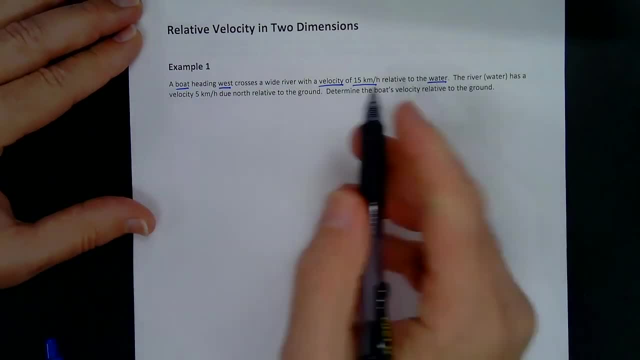 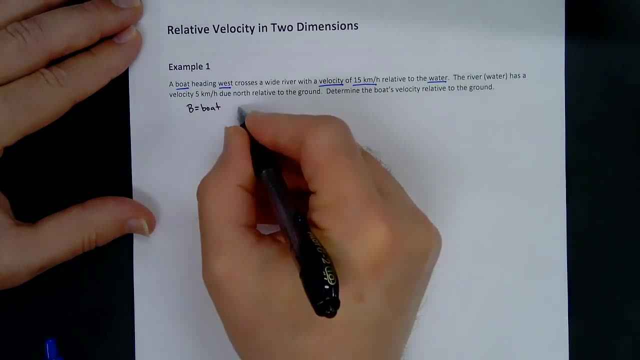 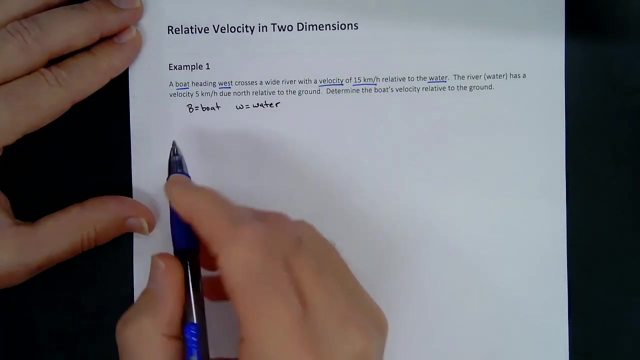 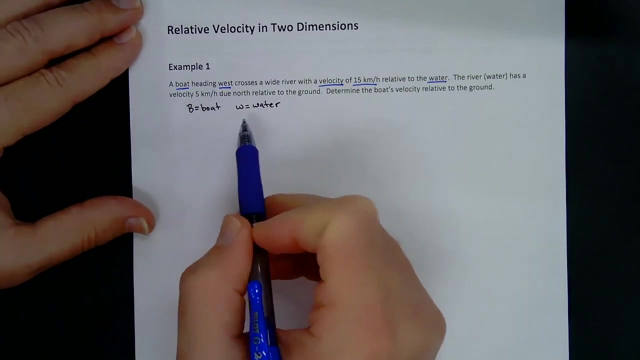 should use subscripts. We're going to use B for boat and W for water, okay, So B equals boat and W for water. So B equals boat and W for water. So B equals boat and W for water, Okay, And so what we have is V sub BW right. So V sub BW- the velocity of the boat relative. 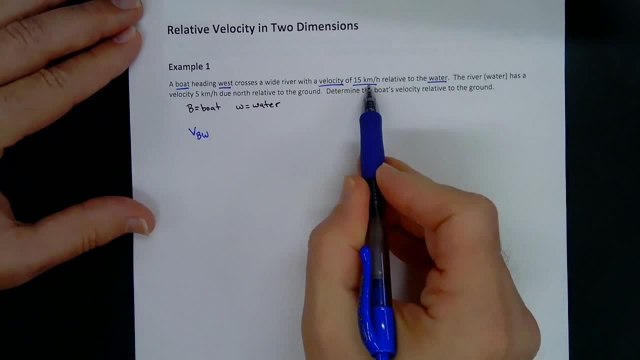 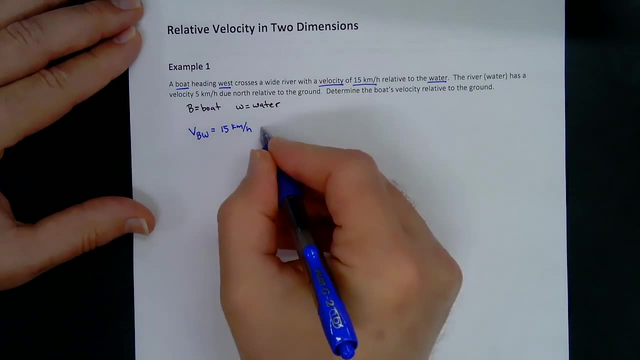 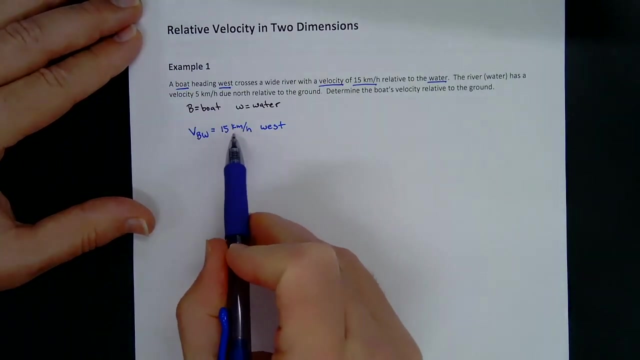 to the water. And we know it's 15 kilometers per hour west. So this is equal to 15 kilometers per hour west. Okay, Now a few things. We have the magnitude of this vector right: It's 15 kilometers per hour. This is the direction. So they don't give you an angle because they say: 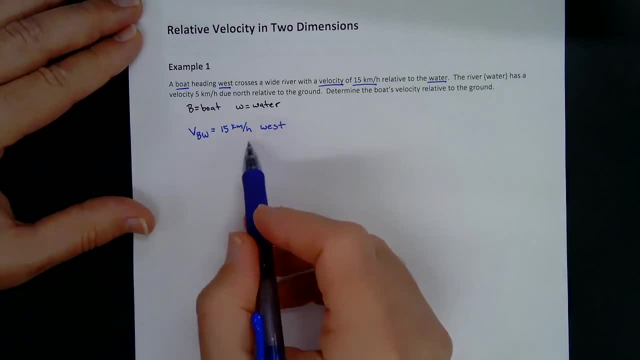 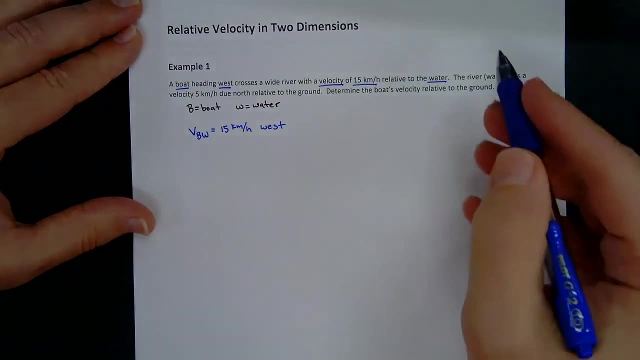 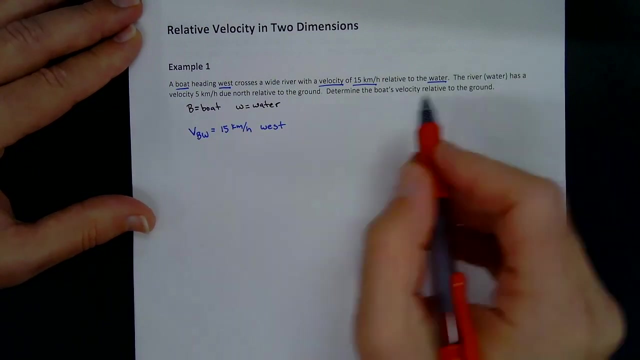 it's west, It's directly west. okay, So we're going to draw a diagram in just a little bit, but I wanted to go over that with you, okay, All right. So then the next thing is: then we have the river, which is also water. has a velocity of five kilometers per hour due north, relative to 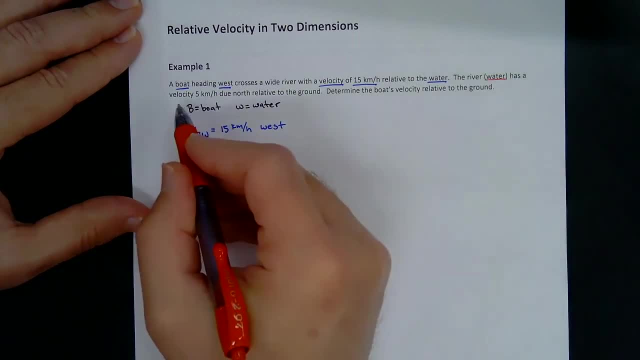 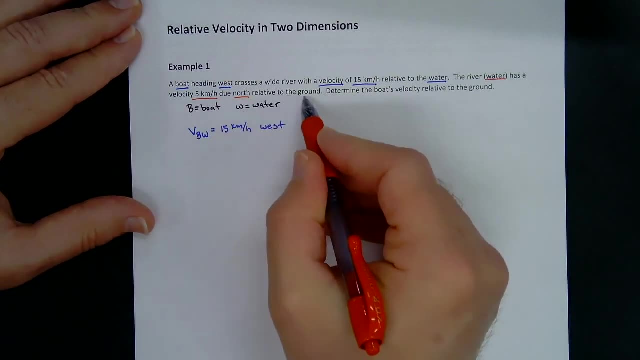 the ground So we have water again. right, That's the object And it's moving five kilometers per hour and it's due north, So directly north, and it's relative to the ground. Okay, So we're going to use- we're going to use- G for ground. 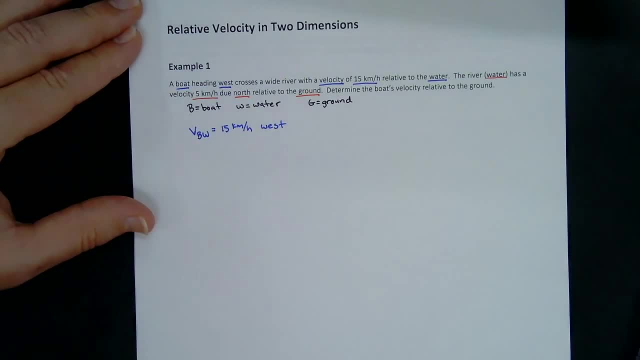 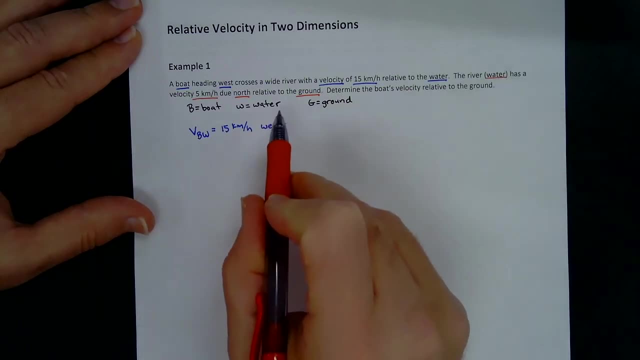 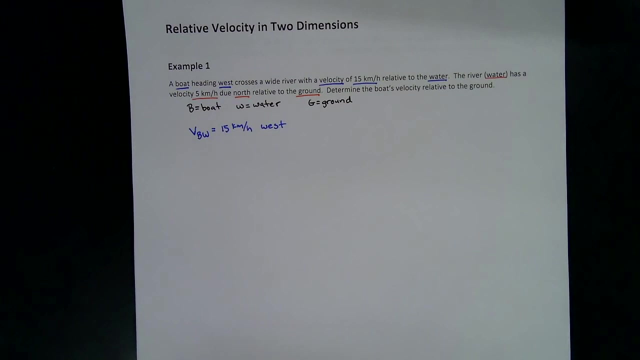 Okay, So what this is giving us is it's V, the velocity of the water with respect to the ground. Now, so the ground is like you think about a river. okay, The river is flowing at a certain velocity and it's relative to like underneath there's ground underneath that river, right? 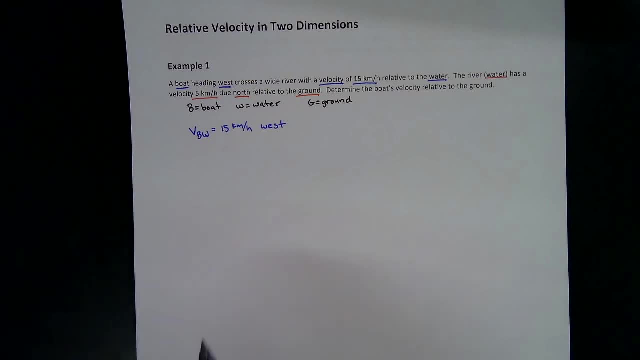 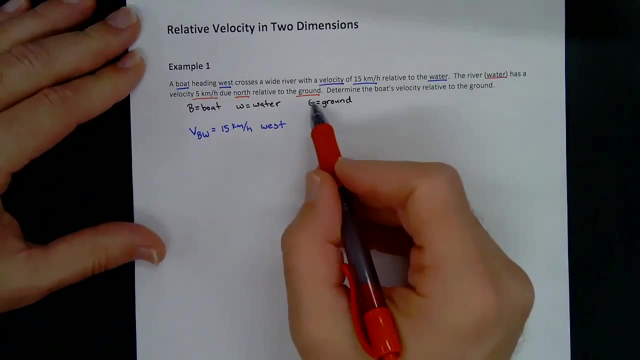 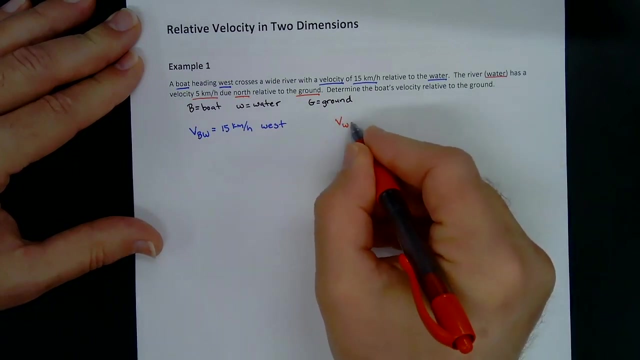 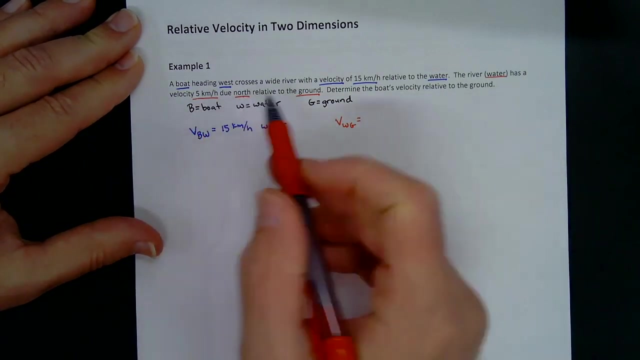 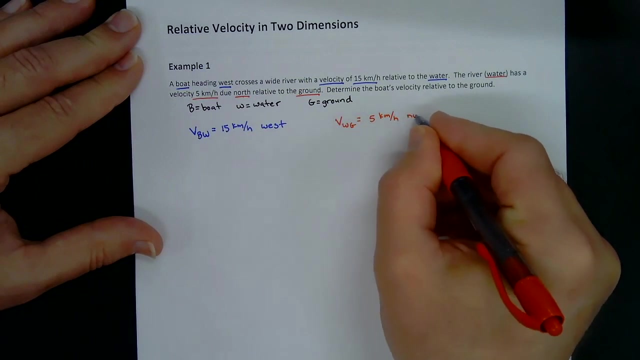 So that water is going across the ground and it's going across the ground at this speed, in this direction, Okay. So this is the velocity of the water relative to the ground. So this would be V sub W, G. Okay, And what we know about that is that it's five kilometers, five kilometers per hour due north. So five kilometers per hour due north, Okay. 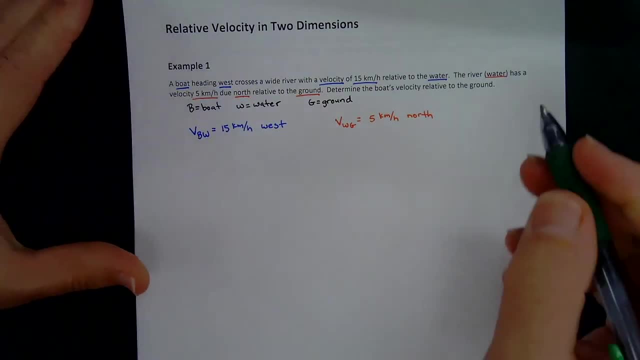 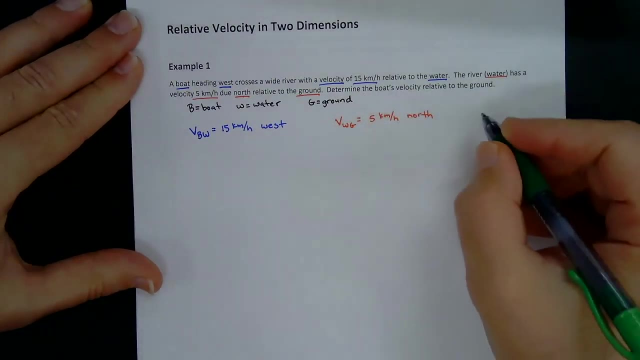 And then what I'm going to do is I'm going to in green, I'm going to draw in. okay, what are we trying to find? We're trying to determine the boat's velocity relative to the ground. So we want to find, okay, V sub and the boat relative to the ground. 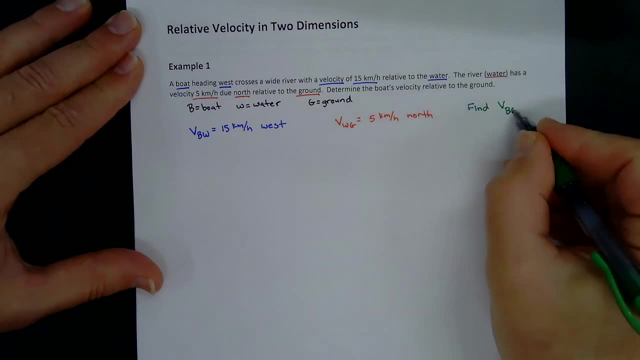 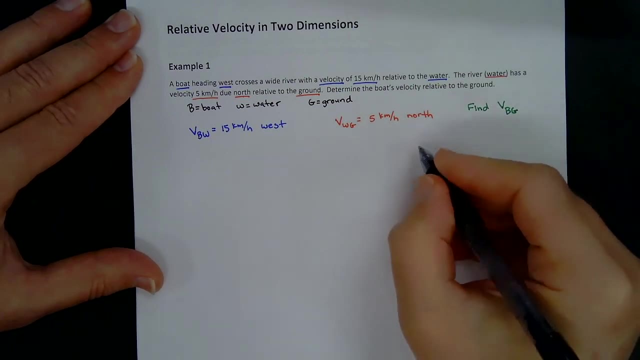 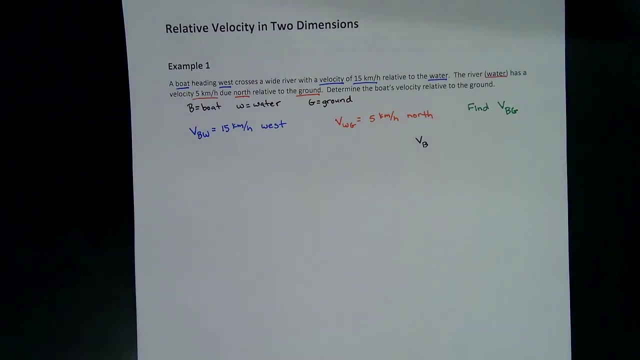 So we want to find V sub B, G. Okay, The velocity of the boat relative to the ground. So we got to write an equation, Okay. So our equation is going to look like this: Okay, The velocity of the boat relative. yeah, I meant to do green. Hold on a second, guys. 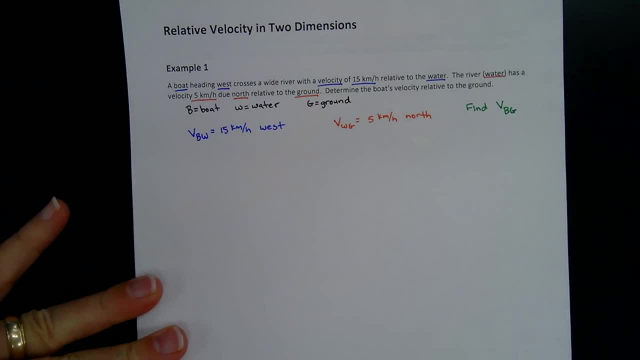 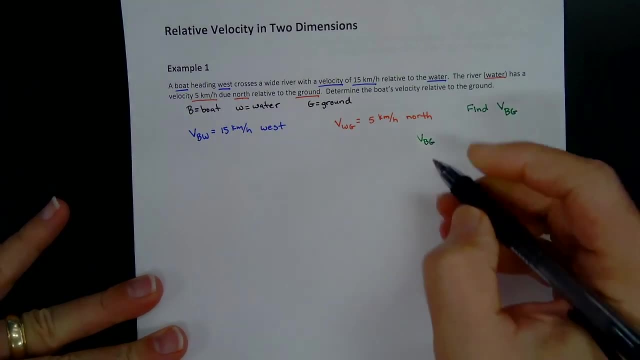 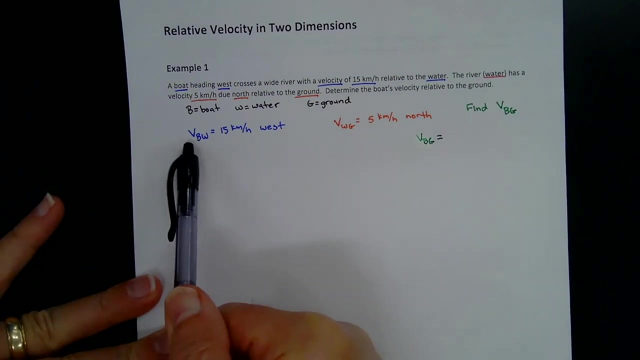 I'm going to erase this and start over again right here. Okay, So I want this to be V sub B, G And this is going to equal. okay, so we can start. we want to start with B. Remember this, We can relate, we can have. we have the velocity of the boat relative to the water. 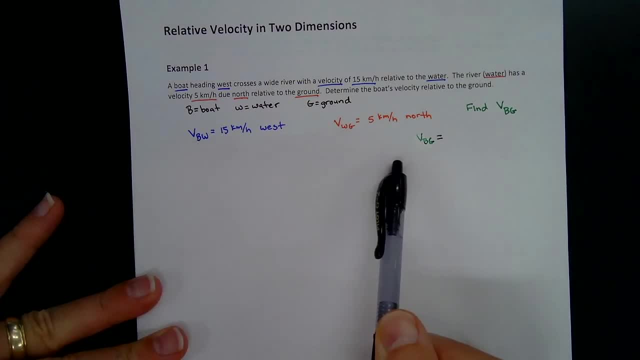 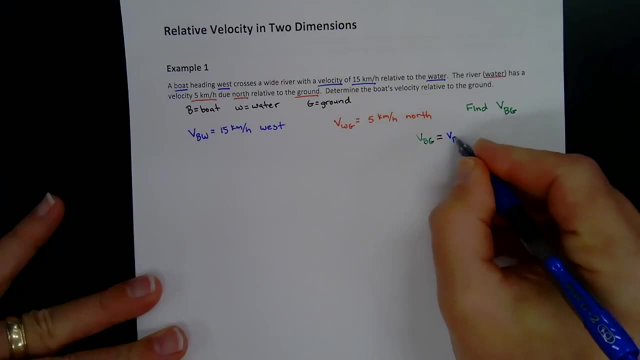 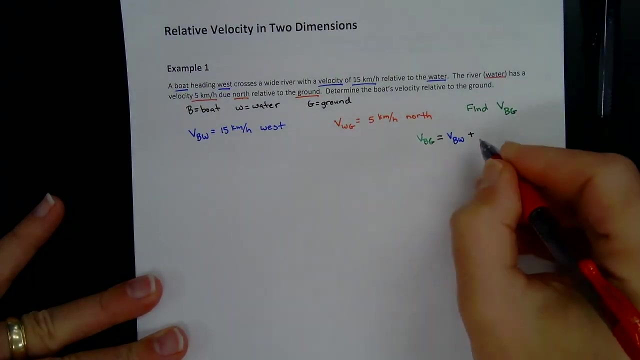 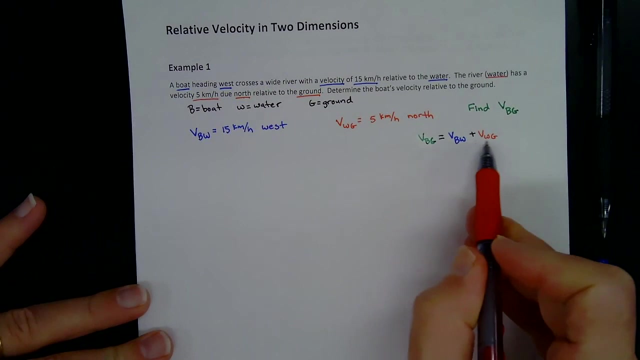 And then the wall. okay, water relative to the ground. So that would give us the velocity of the boat relative to the ground. So this is going to be V sub B- W plus, and then V sub W- G. Okay, But these are vectors, right? So we need to add these two vectors And if we add these two vectors, we're going to get this one, Okay. 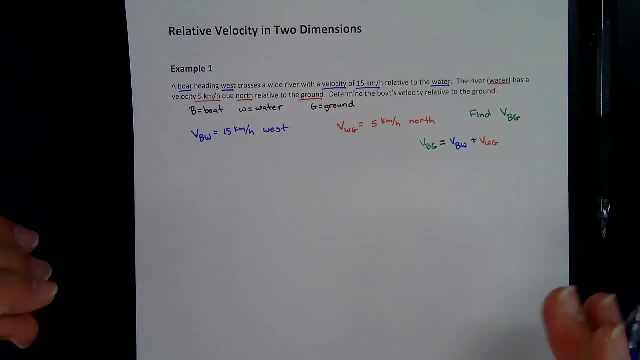 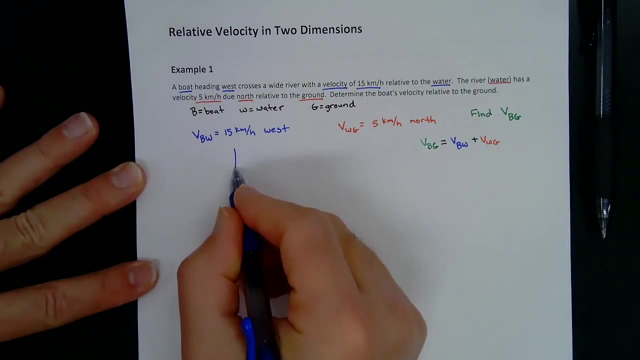 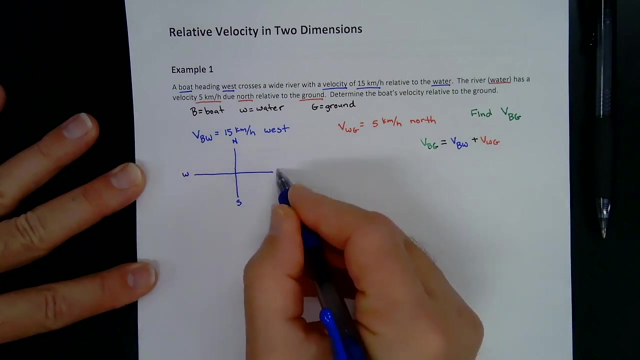 So to do this, this is a fairly- this is actually a fairly simple problem. Okay, The direction of this: we know we're going 15 kilometers per hour and we're going west, So that would look like this: So I know this is north, this is south, this is west and this is east, And I'm going west, I'm going in this direction right, And because I'm going in that direction, that's negative: 15 kilometers. 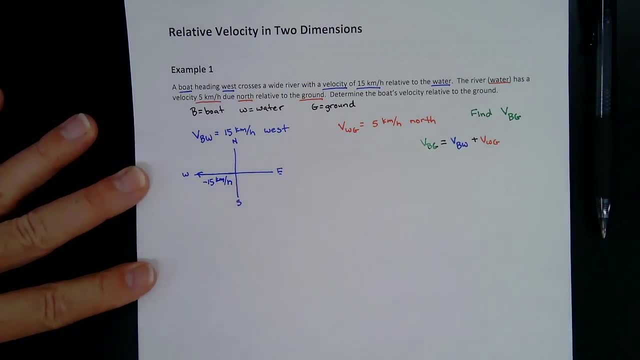 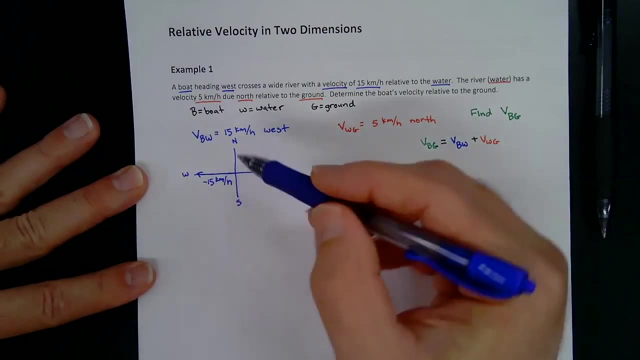 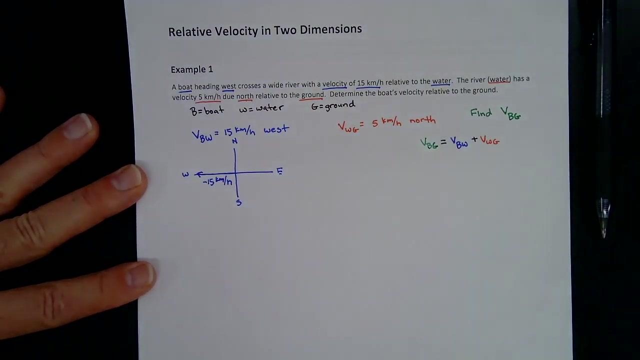 Per hour. Okay, Okay, So what we have is because of this, because it's going directly west. we have a horizontal component to this vector but no vertical, So we're going to use the sub X and sub Y to show the horizontal and the vertical. Okay, so this is V sub B, W, X is equal to negative 15 kilometers per hour. 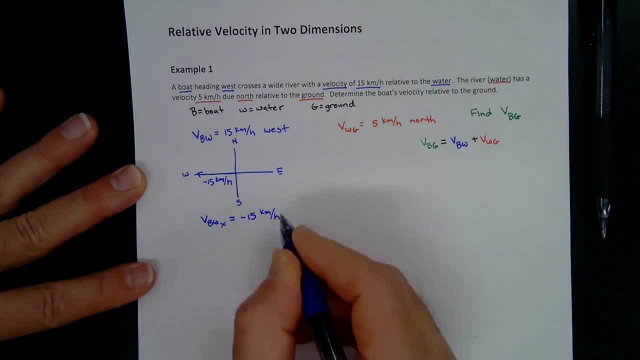 15 kilometers per hour. That's the horizontal component, And then the vertical component. we're going to label V, sub B, W Y, And that is, there's no vertical component, So that'd be zero kilometers per hour. Okay, so then back over here. Okay, so now we need to do this one, So this vector. 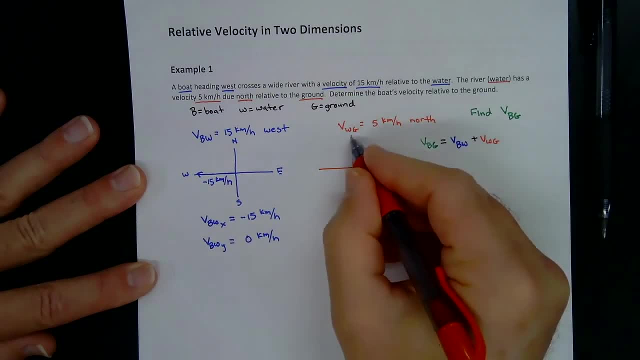 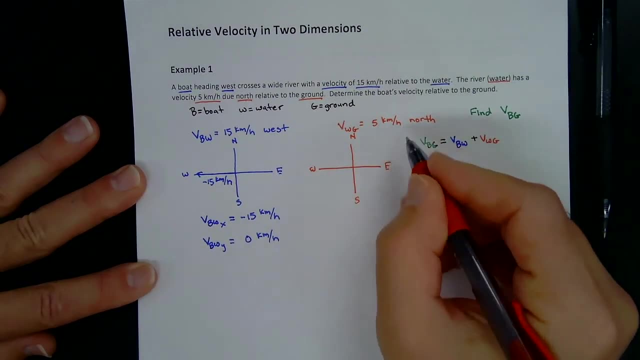 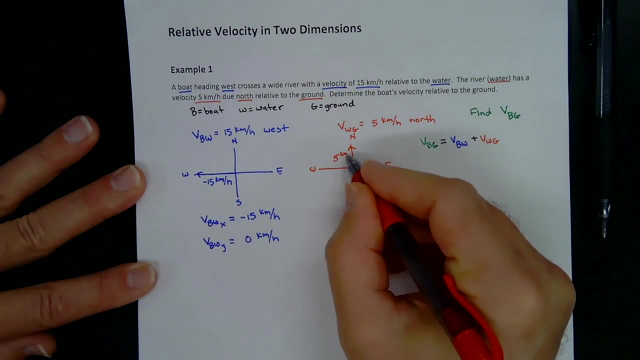 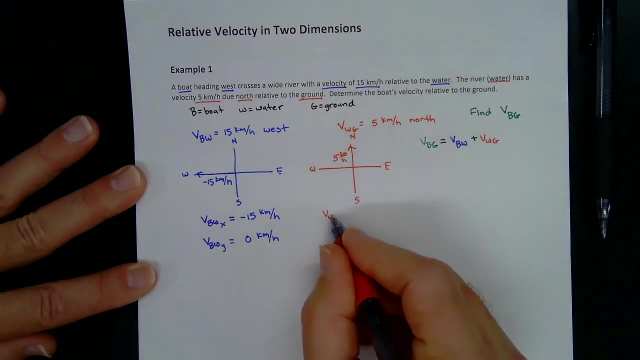 Is five kilometers per hour north. So again, this is north, This is west. I almost wrote south there, This one's south And this one's east, And we're going five kilometers per hour north. So that'd be in this direction And it'd be positive because we're going up. So five kilometers per hour. So that means V sub W, G, X is equal to well, we didn't go horizontal. 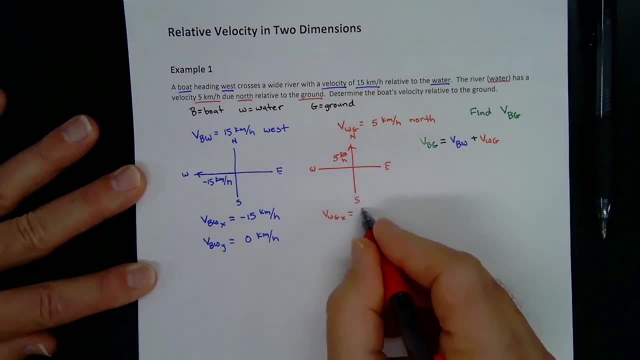 Horizontal at all right. All it's going is vertical. So that means this one is zero kilometers per hour And the the vertical piece it's all vertical right. So that'd be V, sub, W, G, Y And that would be positive five kilometers per hour. 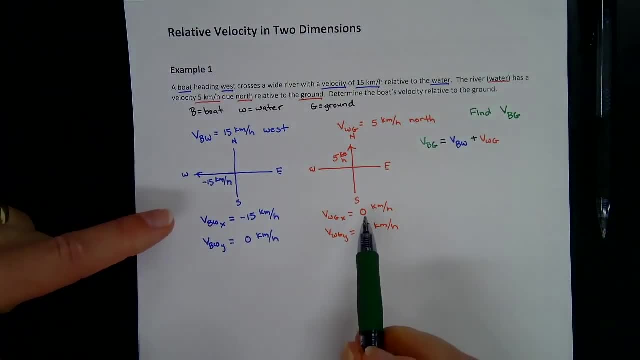 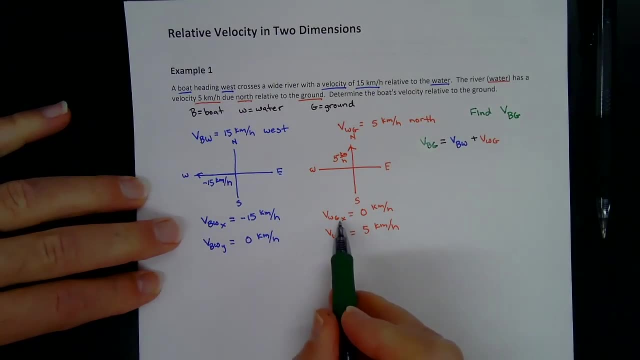 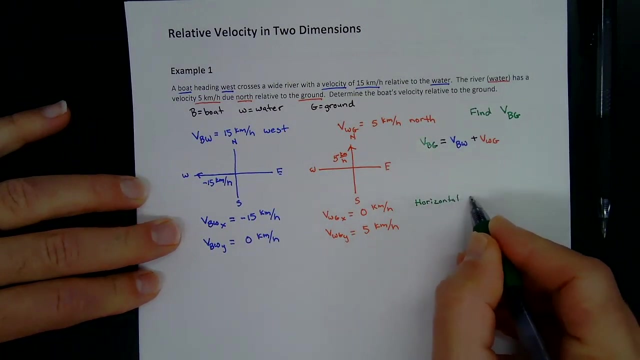 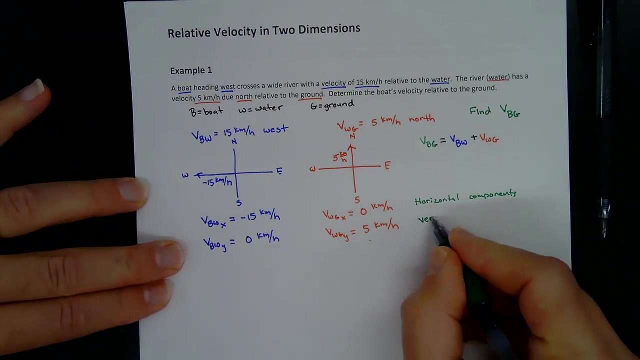 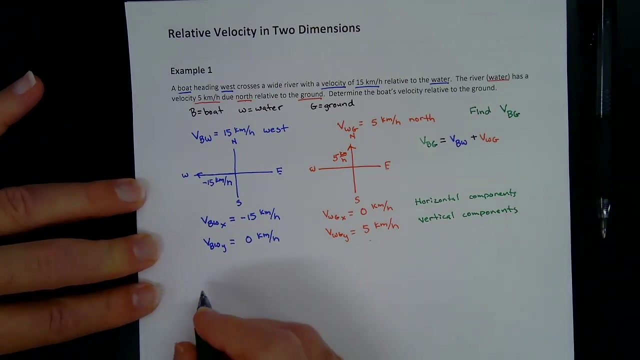 Okay, so we need to add these two together in order to get the V sub B G right. So we need to find the horizontal components right. These are the horizontal components And then these are the vertical components. Okay so, V sub B G. 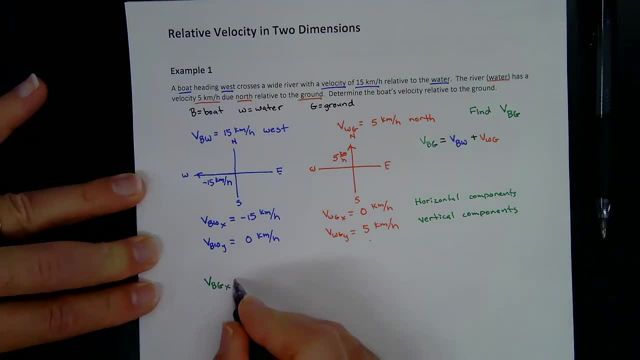 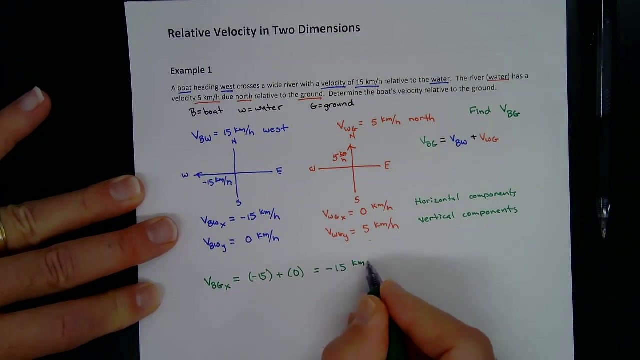 X, the horizontal component to it would be negative 15 plus zero, And that would be in kilometers per hour. So that'd be negative 15 kilometers per hour, And V sub B, G, Y, the vertical component would be zero plus five kilometers. 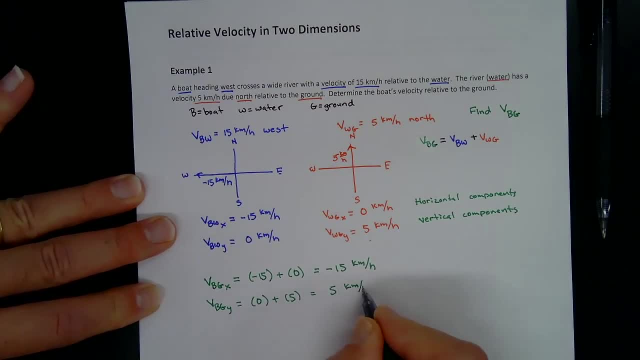 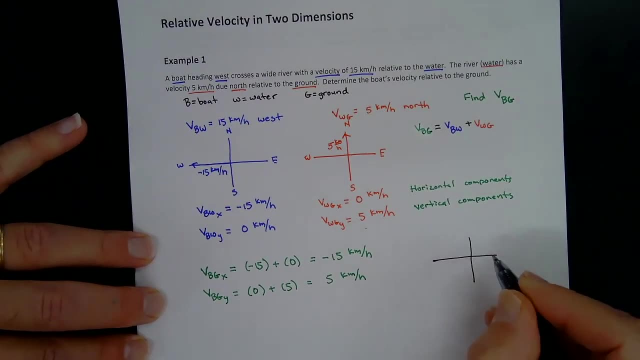 Which would give you five kilometers per hour. Okay, so we're going to draw, we're going to draw a diagram. Okay, so we have this And we're going to go. This would be north, This would be south, west and east. 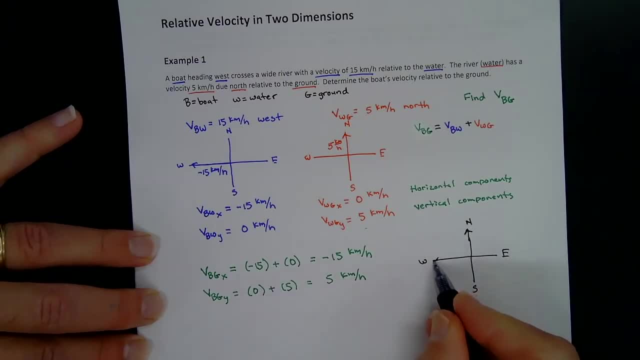 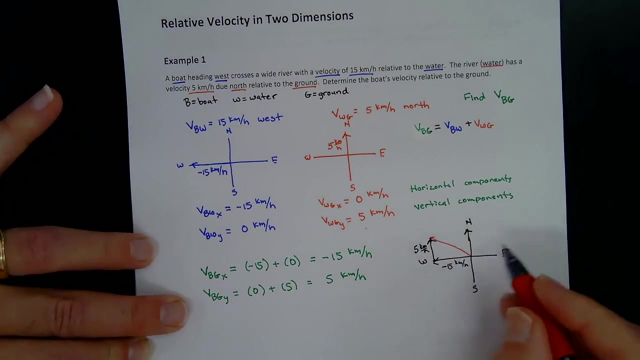 I know I have to go 15 to the left, So this would be negative 15 kilometers per hour. And then I have to go up five, So up five, So I'm going to need to go head in this direction. Okay, so that's my resultant vector. 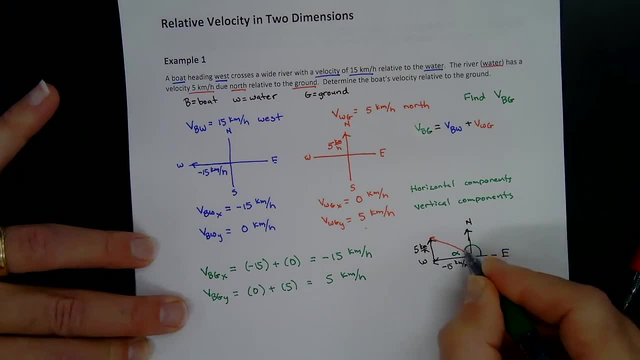 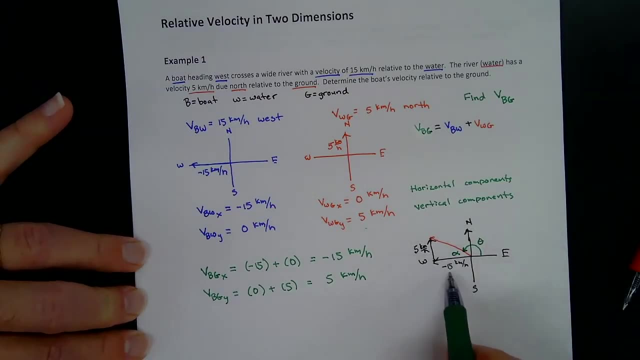 And I'm going to need to find alpha, And I'm going to need to find this angle theta that I rotate, Okay, So let's find, Okay, let's find the resultant vector first. Okay, so that that would be the sub. 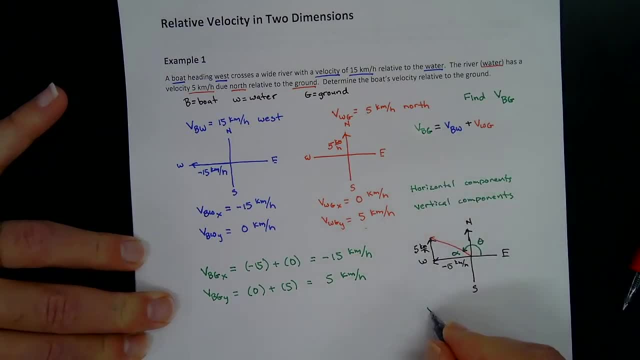 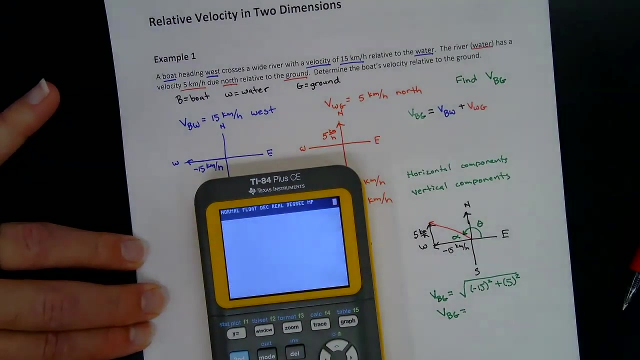 V sub V sub BG would equal the square root of and it would be negative 15 squared plus five squared. So grabbing a calculator And we're going to square root In that second square root And then Negative 15, make sure the negative is in parentheses- and squared and then plus five squared and we get 15.8.. 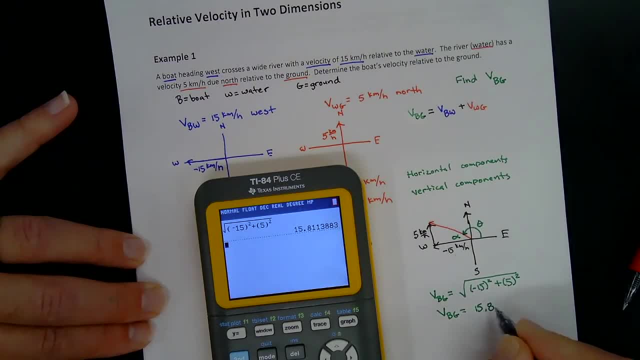 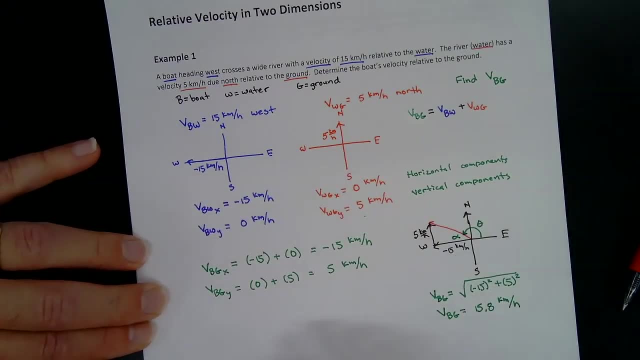 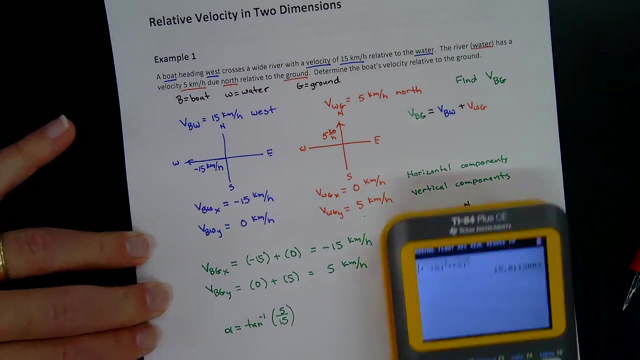 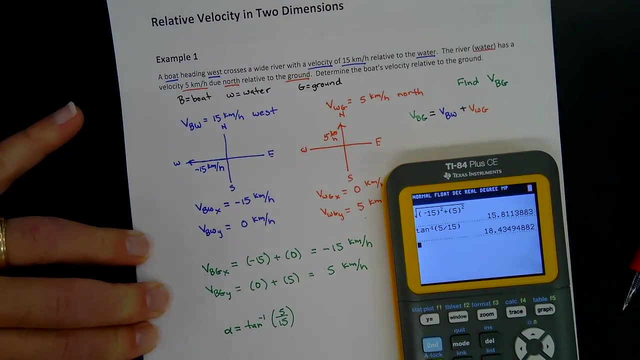 And that'd be 15.8 kilometers per hour. Okay, so now we need to get our angle. our angle would be alpha, and alpha would equal tan inverse of five over 15.. And so second tangent, five divided by 15. And we get 18.4. so that makes it 18 degrees. 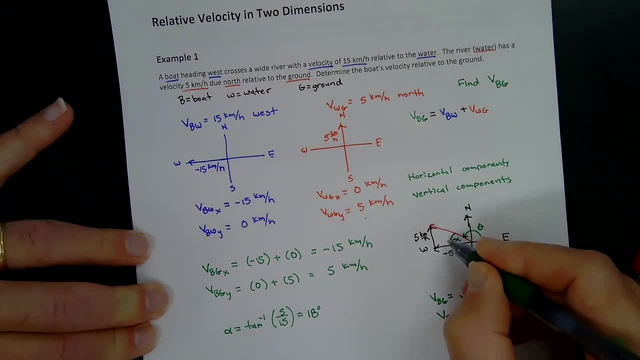 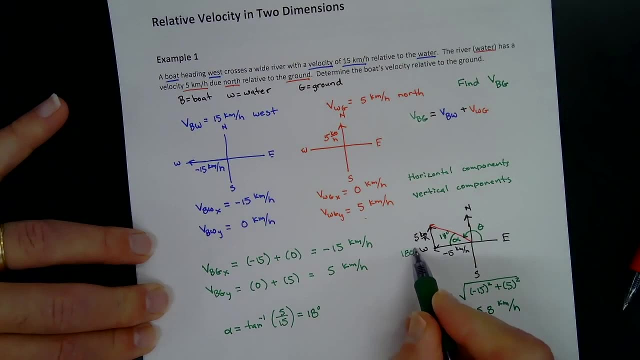 Okay, so that makes this angle right here 18 degrees. All right, so this is 180 degrees right here if we go all the way from here to here. All right, so this is 180 degrees right here if we go all the way from here to here. 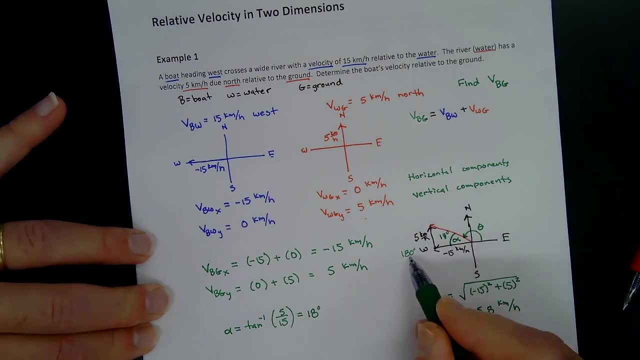 Right, And so this 18 degrees is part of the hundred eight, so we need to use the 180 to figure out theta. So my theta is going to be: We're going to start with 180 degrees, because that's angles connected to 180 degrees. 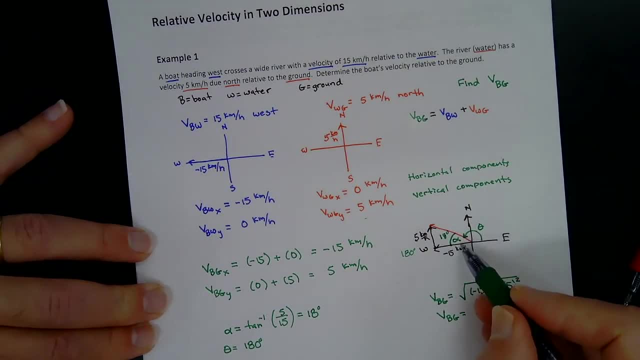 And we got to think, okay, did I go past 180 or did I stop before 180? so I stopped before right? So I'm going to have to subtract the 18 degrees, Okay, and that would give you theta as being 160 degrees. 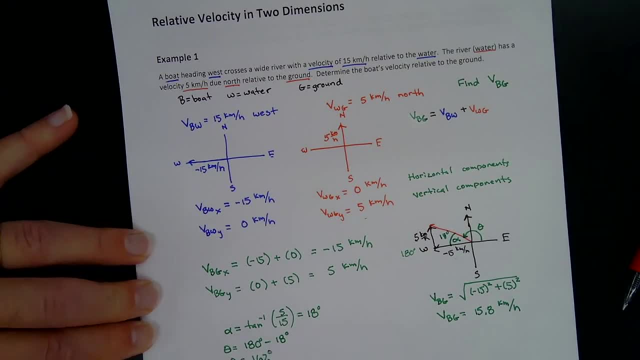 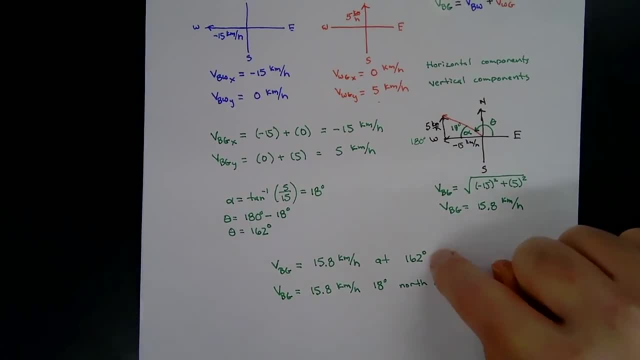 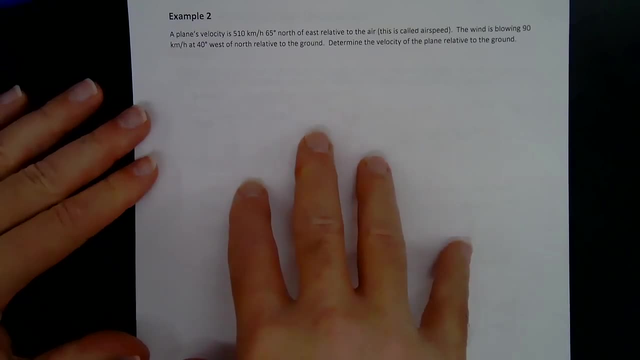 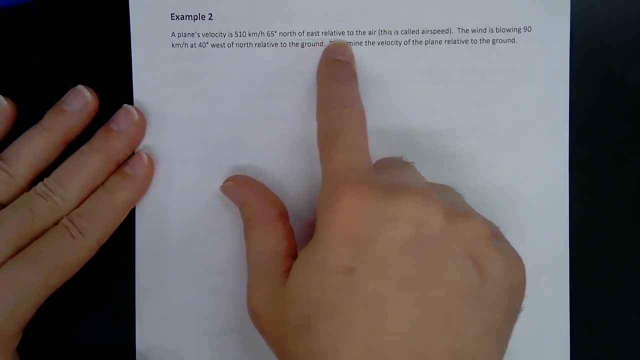 So two ways of explaining it. okay, I prefer this one. okay, because we can use this to find other stuff if we need to. okay, So for this next example, all right, we have a plane's velocity in at 510 kilometers per hour, 65 degrees north of east relative to the air- this is- when its relative to the air- the plane, 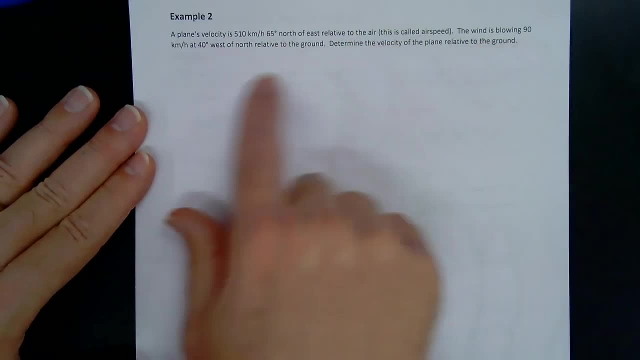 relative to the air. that's called airspeed. okay. And then the wind is blowing 90 kilometers per hour at 40 degrees west of north relative to the ground. All right, so we want to determine the velocity of the plane relative to the ground. 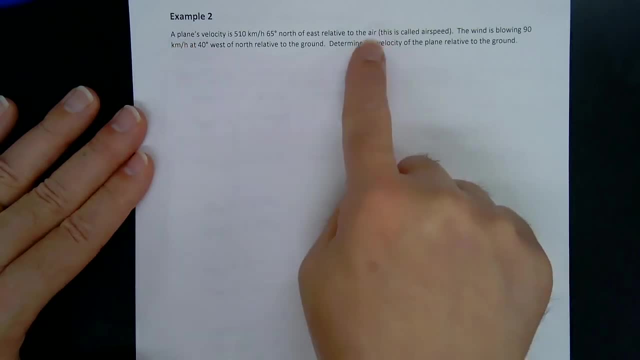 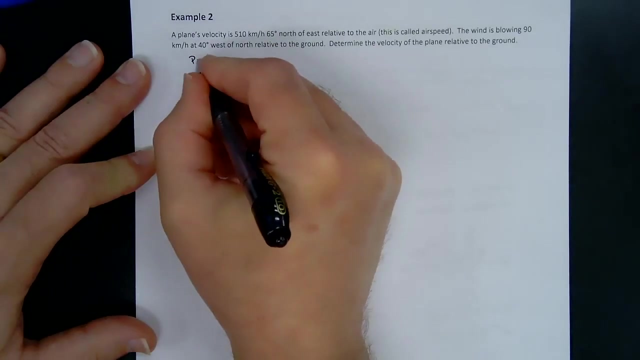 So what we have is the plane, the air, and then we have the air and we have the ground, and then we want to find the velocity of the plane relative to the ground. So we want to. we're going to use P for plane, A for air. 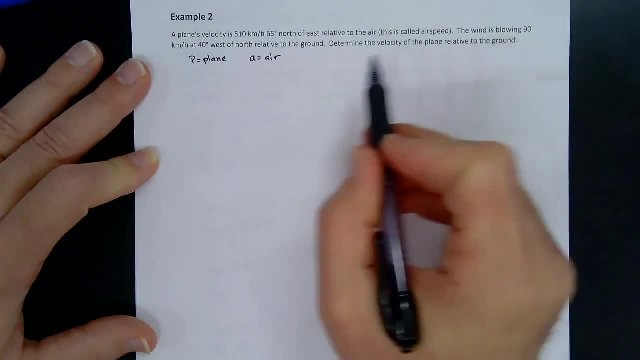 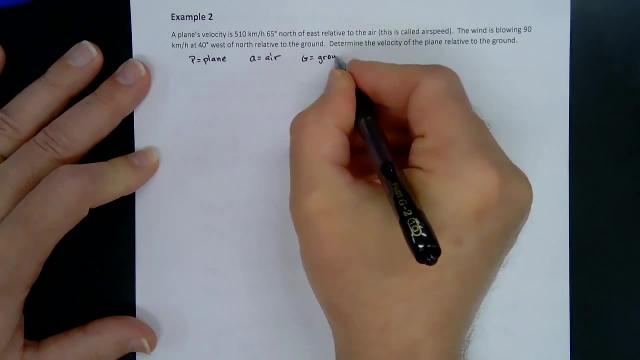 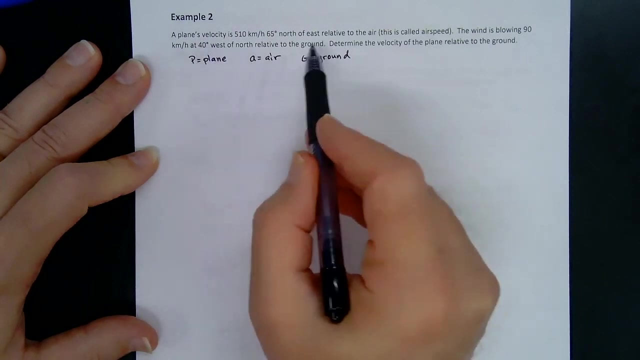 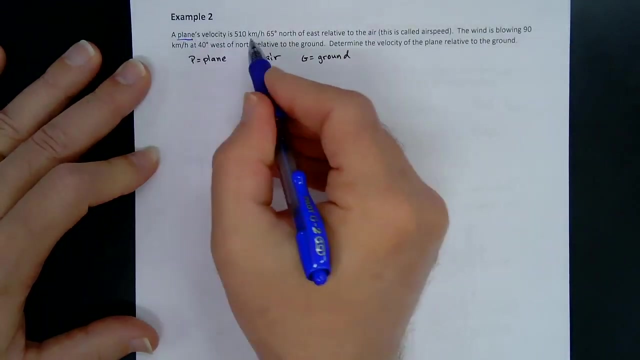 Or capital A. you can use capital A too, And then I'm going to do G for ground. All right, so what we've been given is V sub PA. So this is the plane: 510 kilometers. This is the direction, 65 degrees north of east. 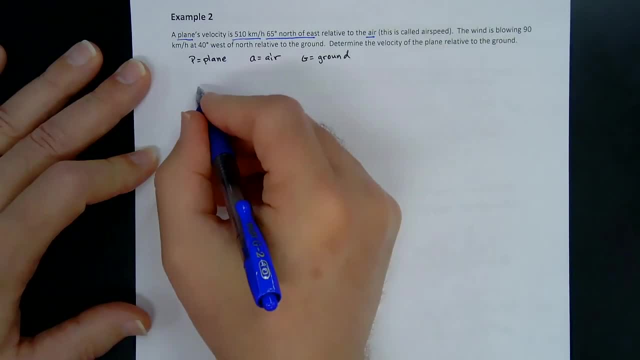 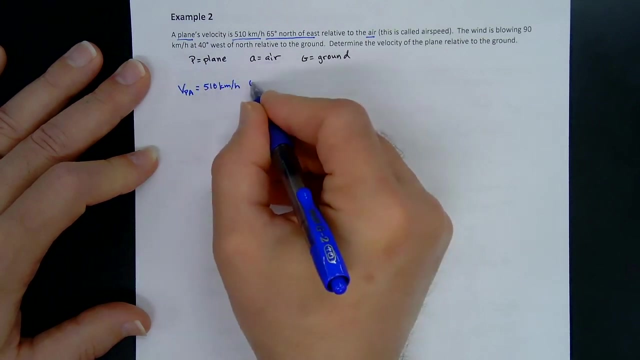 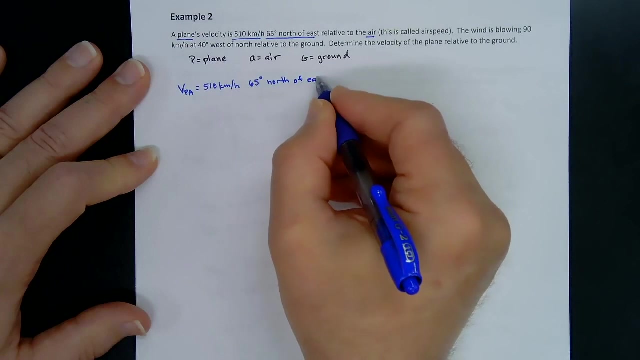 And relative to the air. So this would be V sub and it would be PA. And what do we know about this? It's 510 kilometers per hour and it's 65 degrees north of east. All right, the next velocity is the wind. 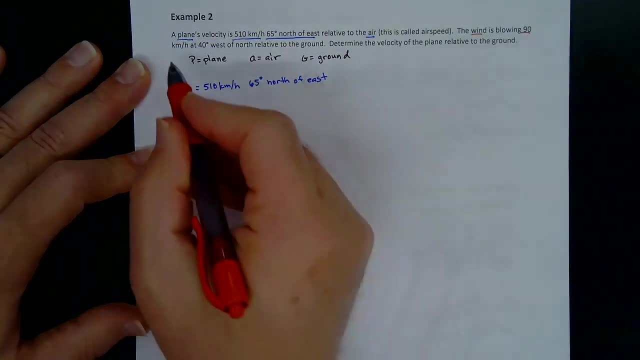 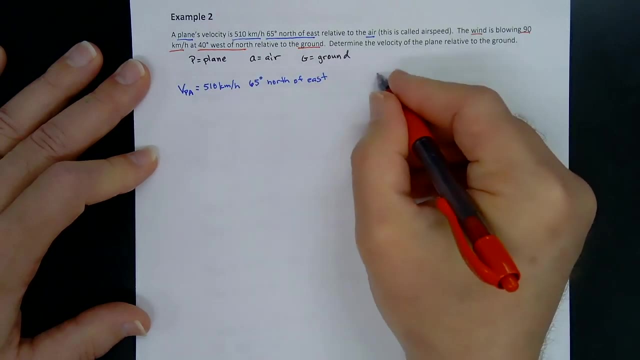 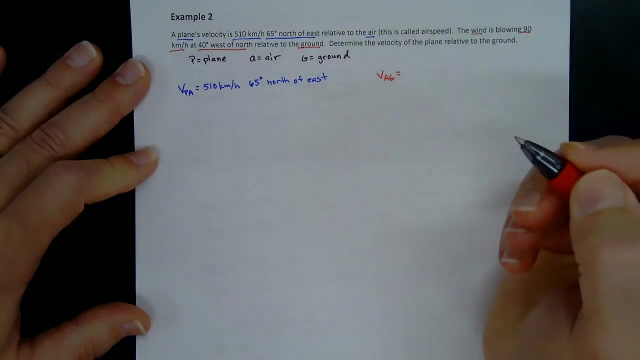 Wind is blowing at 90. So wind is blowing 90 kilometers per hour at 40 degrees west of north relative to the ground. So that would be V sub and it would be AG. Okay, and V sub- AG would be 90 kilometers per hour. 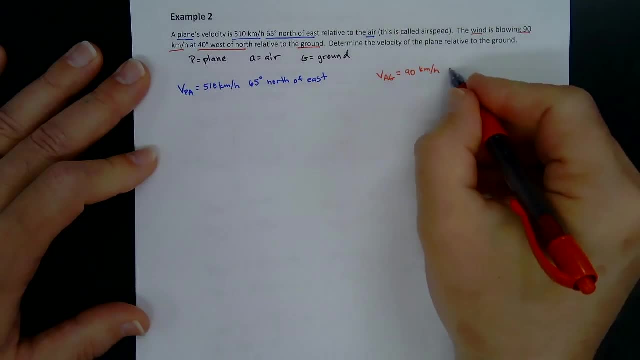 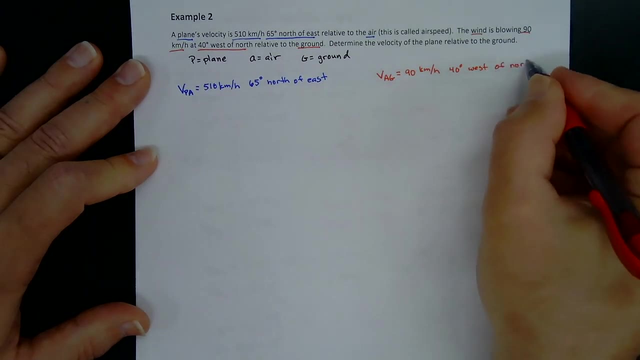 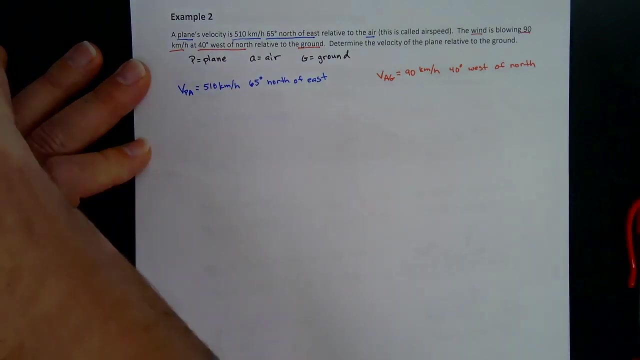 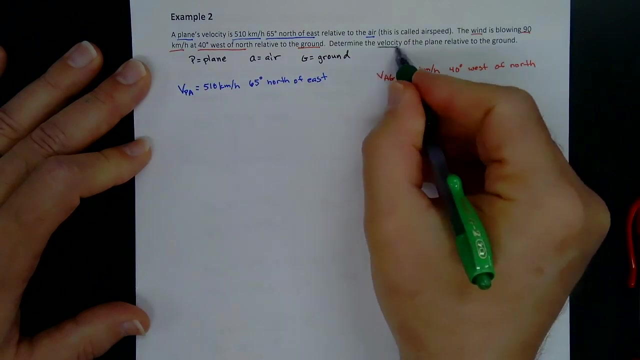 And the direction is 40 degrees west of north. Okay, so all right, and then we want to find. what we want to find is the velocity of the plane relative to the ground. So that would be V: velocity of the plane relative to the ground. 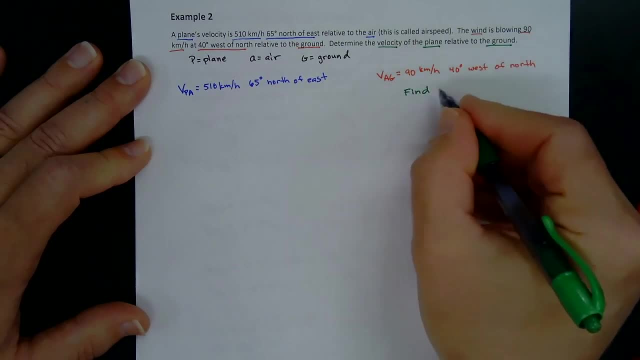 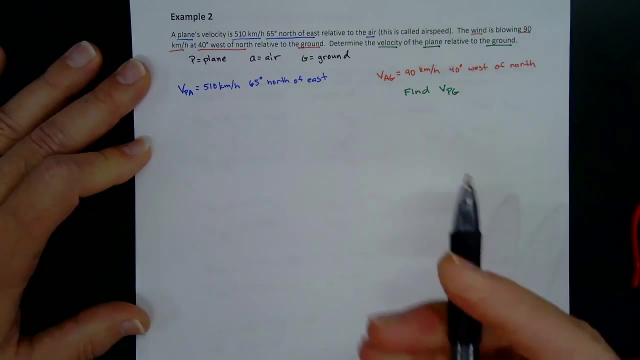 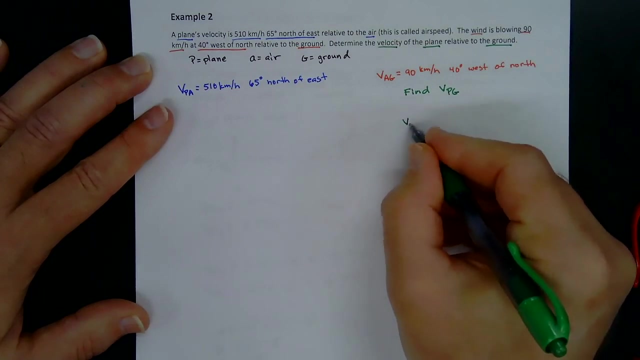 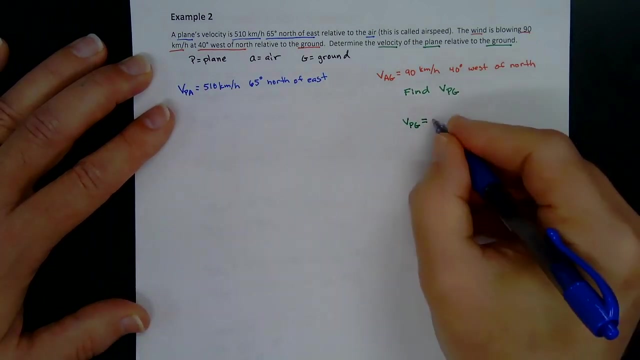 So we want to find V sub. Okay, so all of these are related, Okay, so we got to start. if we want to find V sub PG, That's going to equal velocity of PA, And we're doing this with one dimensional. it works in two dimensional too. 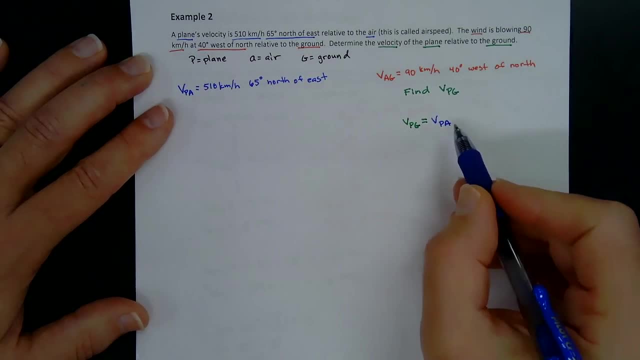 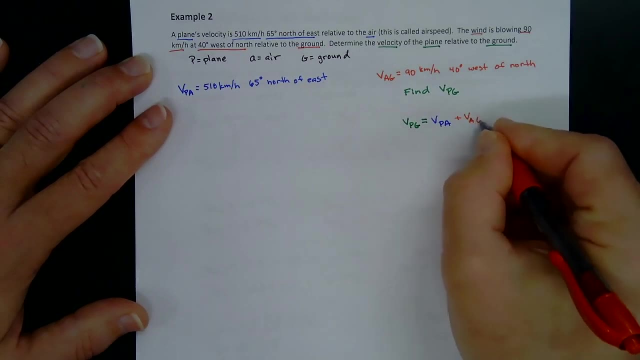 So the velocity of the plane relative to the air, and then we're going to start with the air relative to the ground right And we have that So plus the velocity of the air relative to the ground. So if we add these two vectors, we're going to get this vector. 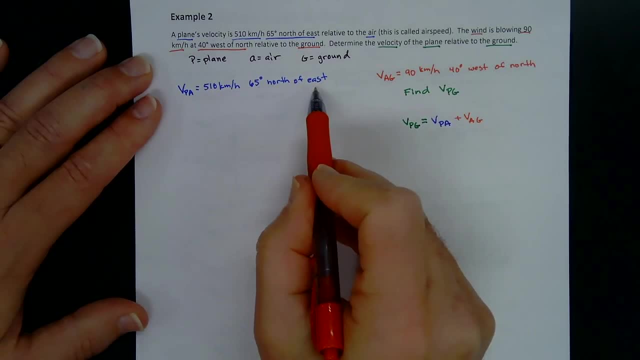 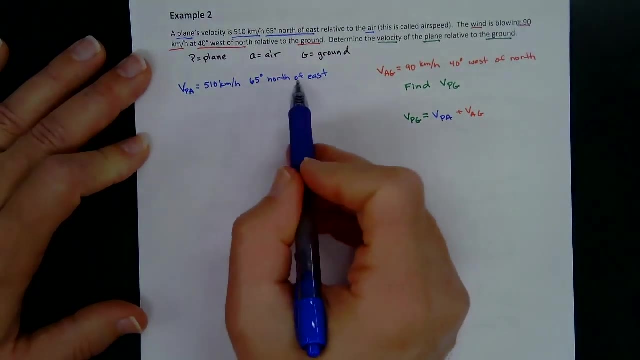 Okay, and to add these two vectors, I got to find the horizontal piece here and vertical piece and the horizontal piece here and the vertical piece. Okay, but the problem is it's it's a verbal description of the direction, right. 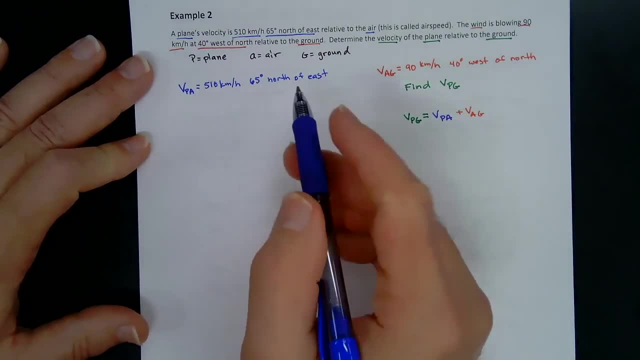 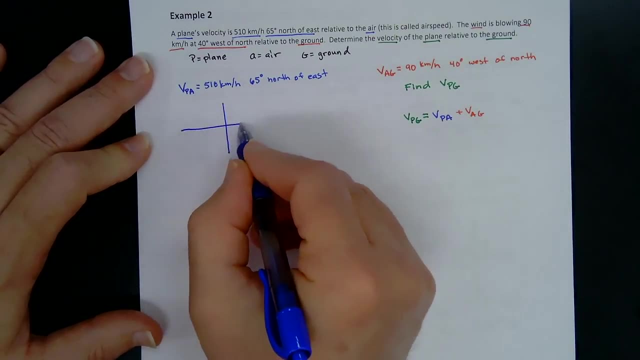 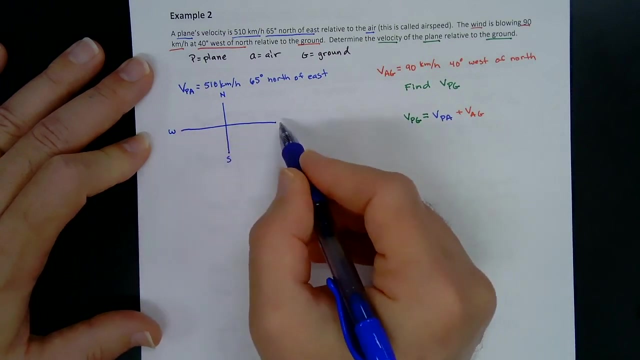 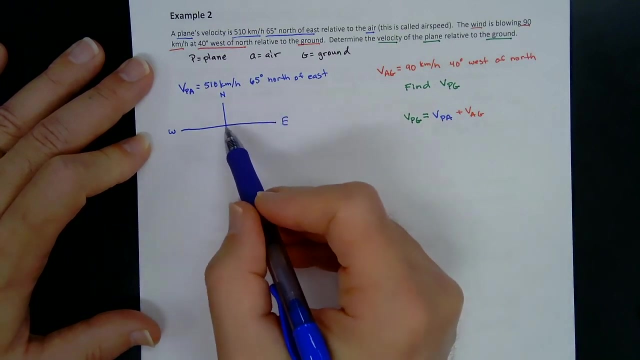 Not an angle. Be great if we had the angle right. In fact, that's what we need. Okay, so we're going to draw a picture of this and we're going to translate it into An angle. okay so, so this is north and this is south and this is west. today I'm having a tough time: north, south, east, west. I don't know if you've noticed that I have to think: okay, so we're doing 65 degrees north of east, so that would be in this direction right here. so we're going, we're rotating north from the east. all right, so we're starting east. 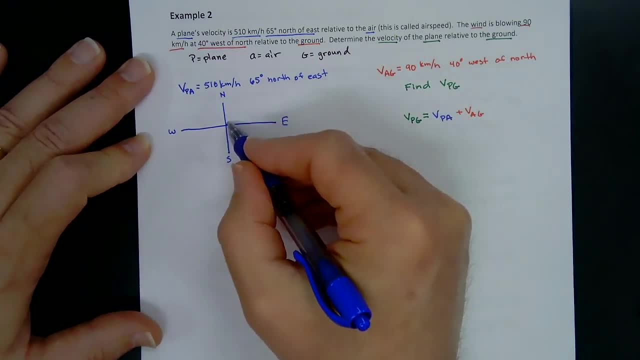 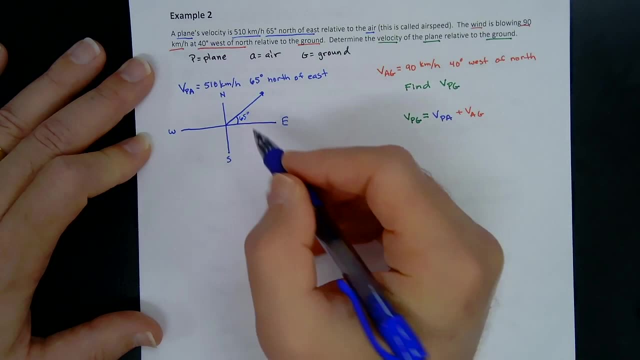 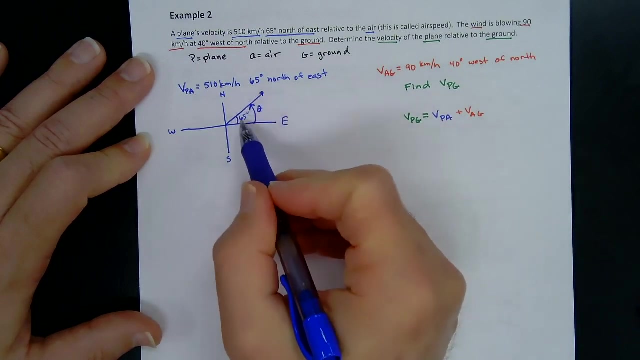 Okay, and we're going to rotate this way, and it's 65 degrees, So this angle is 65 degrees. Well, that's also my angle of rotation data Right? So in this, when it happens to be in this quadrant, the angle that I give you here, Okay, and the angle of rotation happened to be the same thing. Remember, this angle of rotation always has to start on the positive x axis. 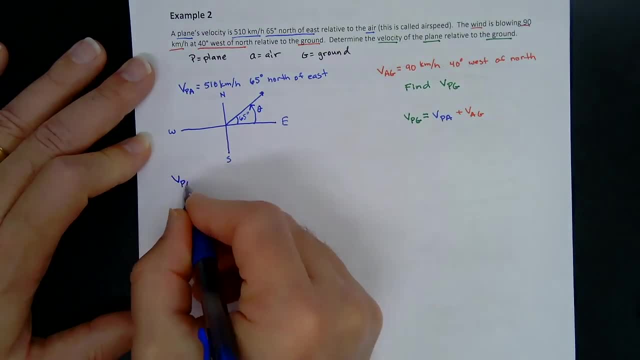 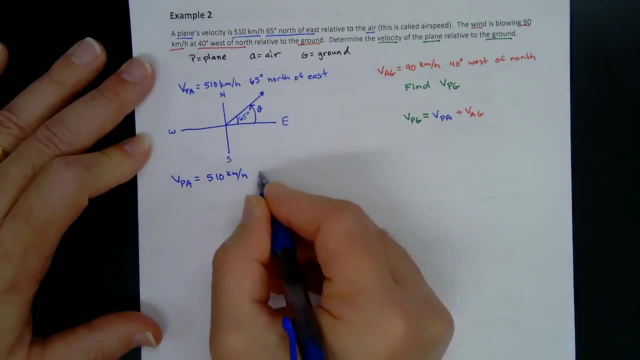 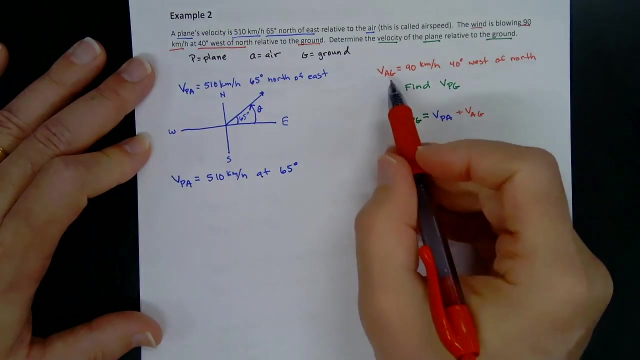 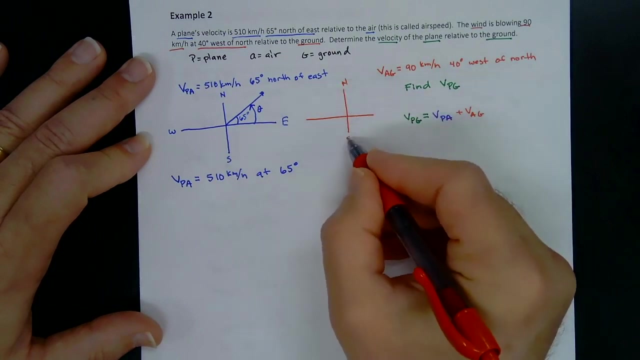 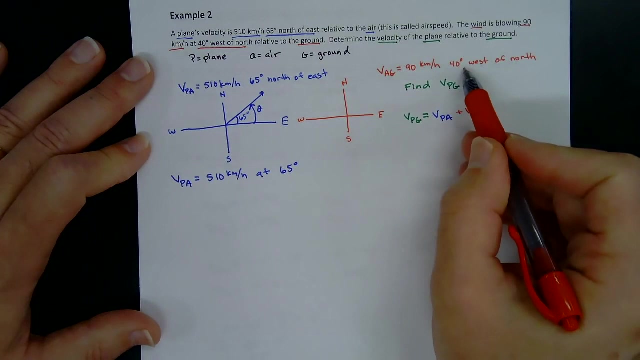 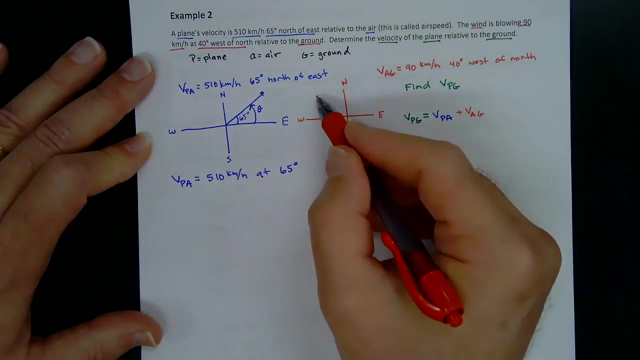 So what we know is V sub PA is equal to. now. we can rewrite it as 510 kilometers per hour at 65. degrees. Okay, Now we need to do this one too. Okay, so for this one, Okay, this would be north, this be south, this be west, this be east. and we know it's 90 kilometers per hour, but the angle is 40 degrees west, Okay, of north. so we're starting this time, we're starting north and we're going to rotate 40 degrees, right, so we're rotating this way. 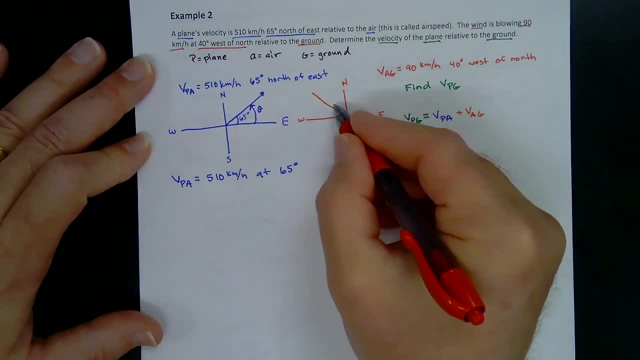 And we know that This angle is 40 degrees. Now that's attached to this one that's 90 degrees right, And so my angle of rotation. I'd have to start right here and go all the way to here. So notice, I've rotated past the 90 right, and how much more that one. 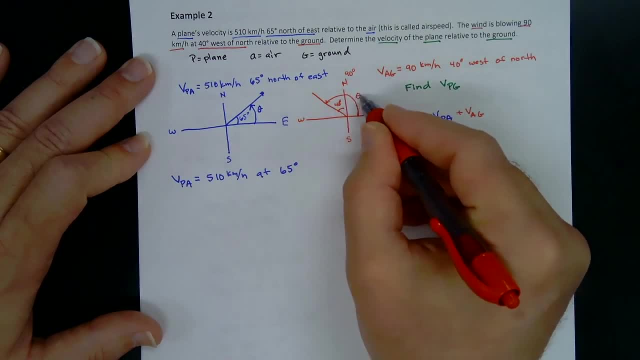 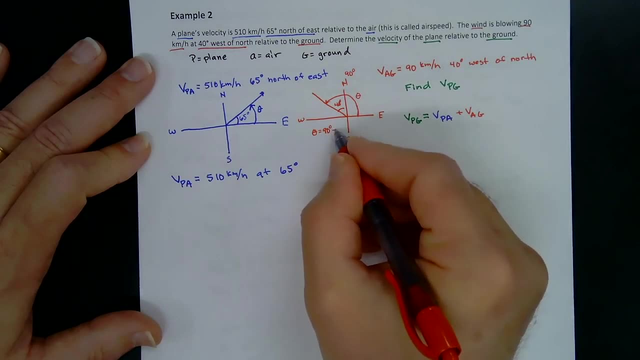 So we're going to have to use the 90 degrees to get my angle of rotation theta right, And so my angle theta would be theta. we would take 90 degrees and add the 40 degrees, which gives me an angle of 100. 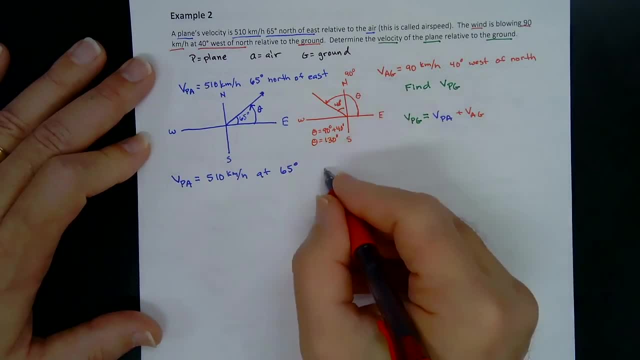 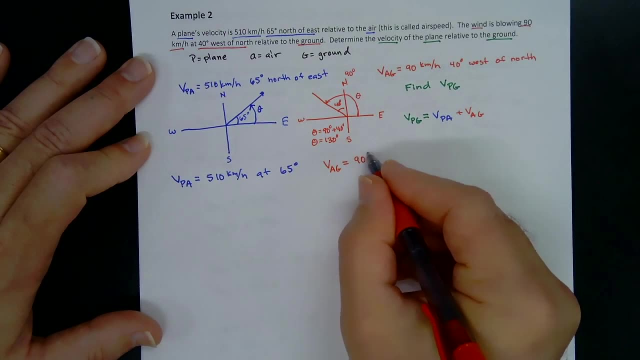 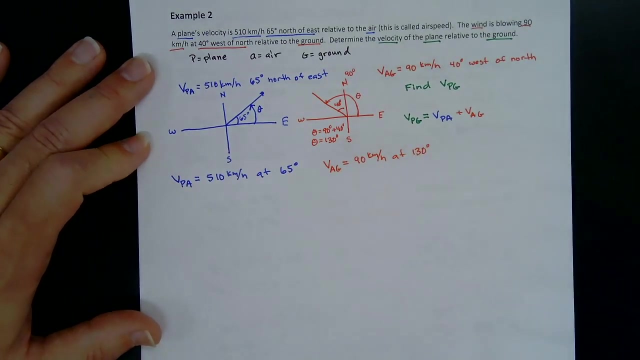 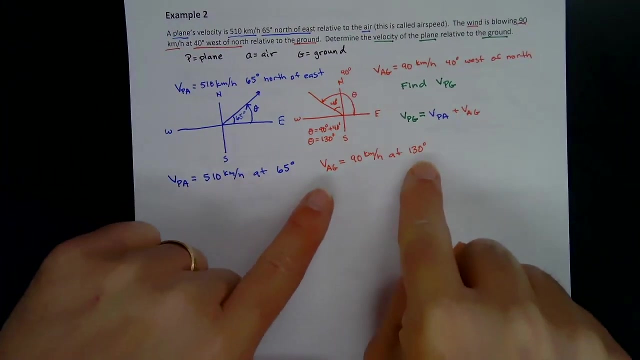 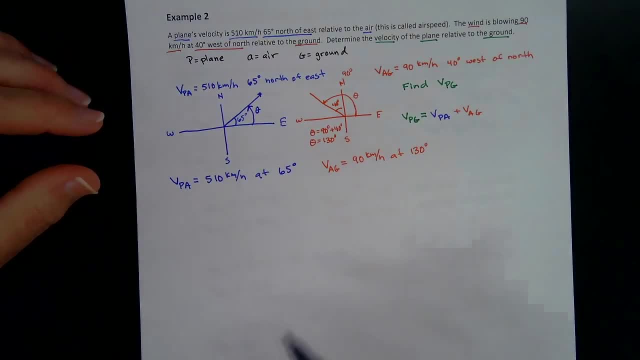 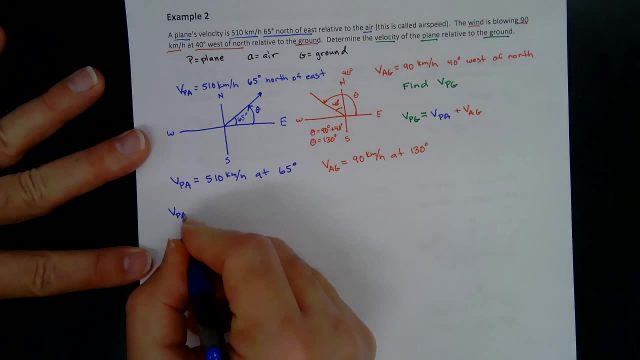 pieces together, and then I'll have the horizontal and vertical components of this vector right here. Okay, So v sub p, v sub p a of x is equal to the 510 kilometers per hour cosine of 65 degrees, and v sub p a x would be 510 kilometers per hour. 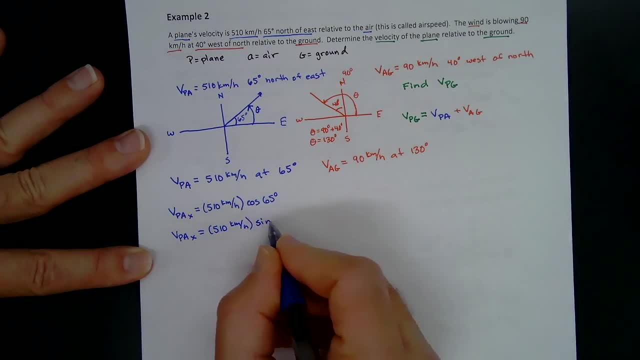 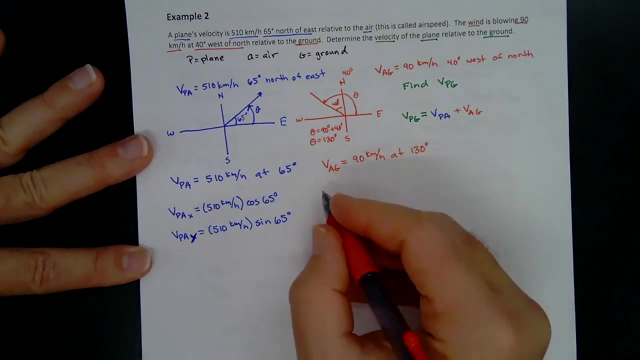 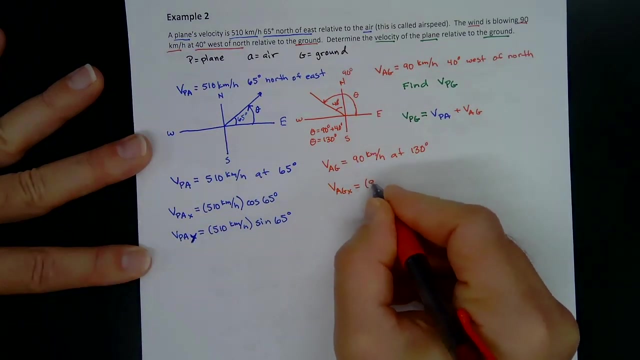 cosine of 65 degrees. So this is the horizontal and this is the vertical. I wrote x and I meant to write y. That should be y right there. Okay, and then this one. we can break it down into the horizontal and vertical components. So v sub a g x is equal to 90 kilometers per hour. cosine of 65 degrees. 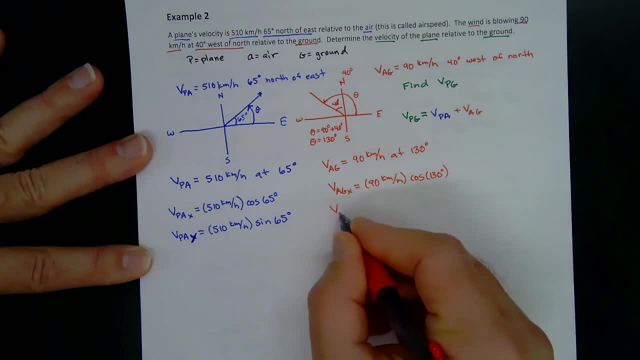 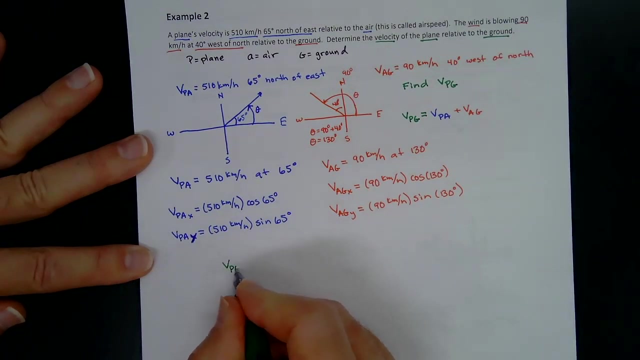 130 degrees And v sub a, g, y is equal to 90 kilometers per hour times sine of 130 degrees. Okay, so that means v sub p, g and the horizontal component- so I'm going to put an x for the horizontal component- is equal to 90 kilometers per hour times sine of 130 degrees. 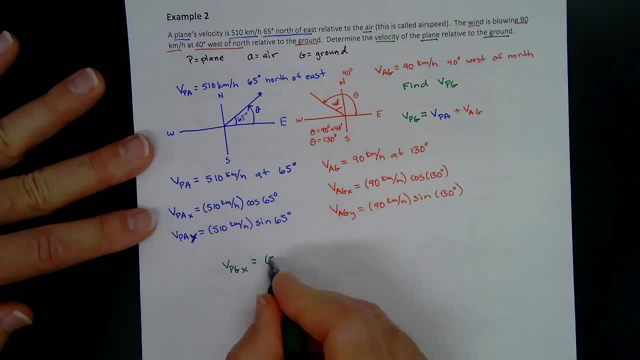 Okay, so that means v sub p, g, x is equal to this horizontal component, which would be 510 kilometers per hour, cosine of 65 degrees, plus this horizontal component, which is 90 kilometers per hour, cosine of 130 degrees. 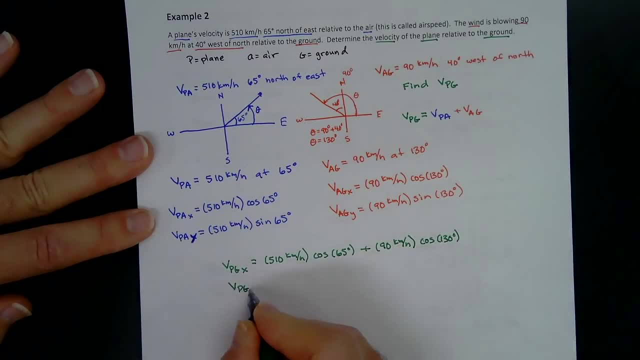 Okay, so that means v sub p g. x is equal to 90 kilometers per hour times sine of 130 degrees. Okay, so this is the vector we're trying to figure out. Okay, I'm going to type this in my calculator. 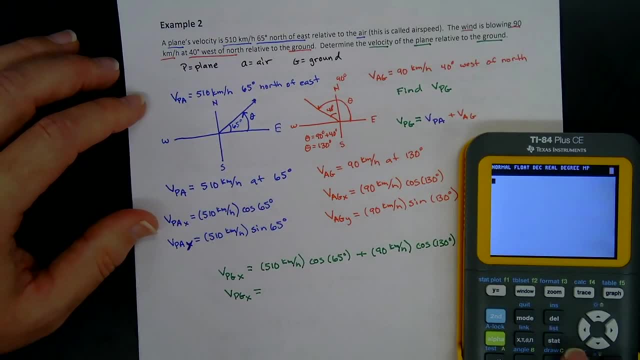 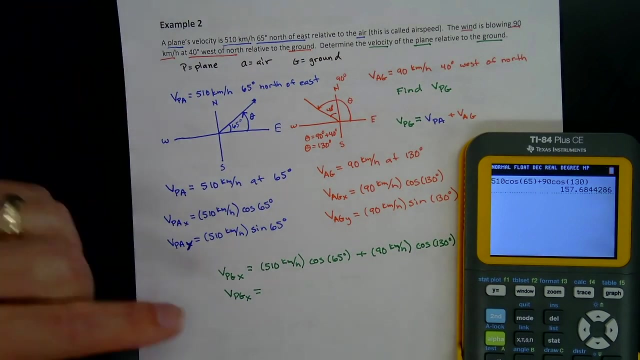 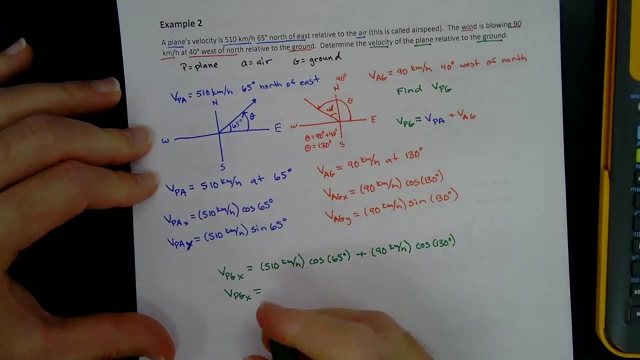 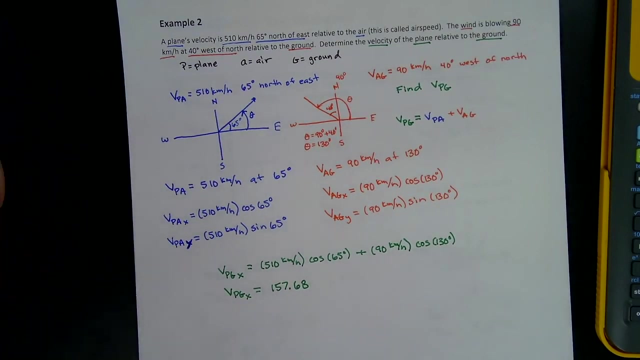 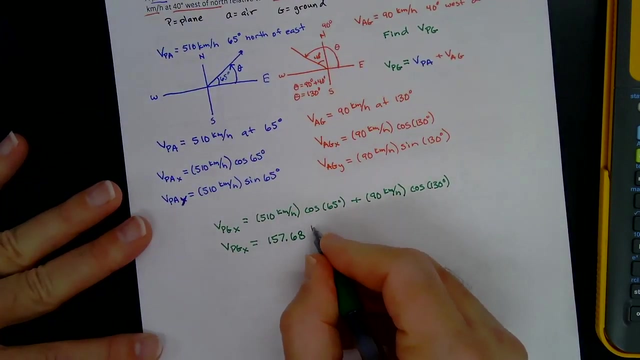 Okay, so 510 cosine of 65, plus 90 cosine of 130.. And we get 157.68.. So the horizontal and vertical components, I want you to round to two decimal places. Okay, so 157.68.. All right, And now we got to figure out the vertical component. Okay, and I should say this is kilometers per hour. 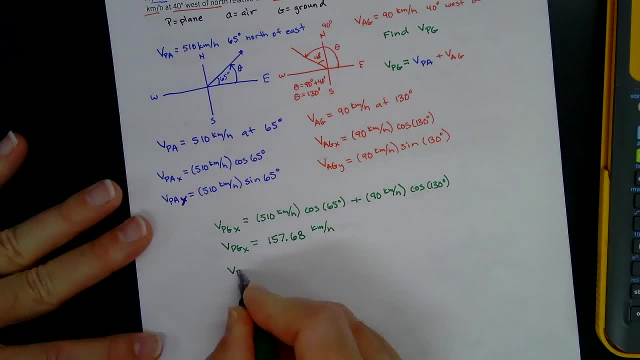 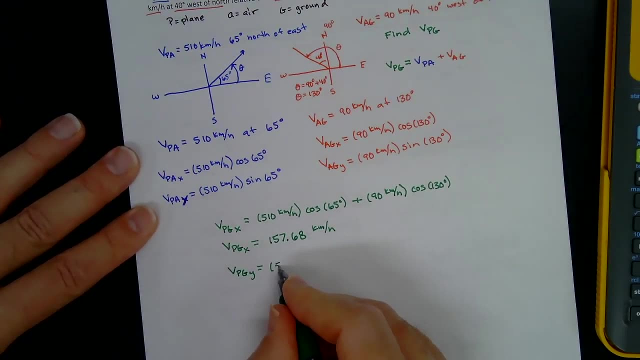 And so now we need to find v sub p g y. So that would be this horizontal component, or horizontal vertical, 510 kilometers per hour, sine of 65.. Plus 90 kilometers per hour Sine of 130 degrees. So that makes v sub p g y equal to. 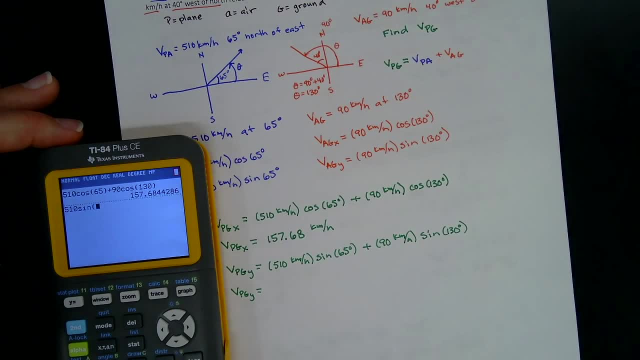 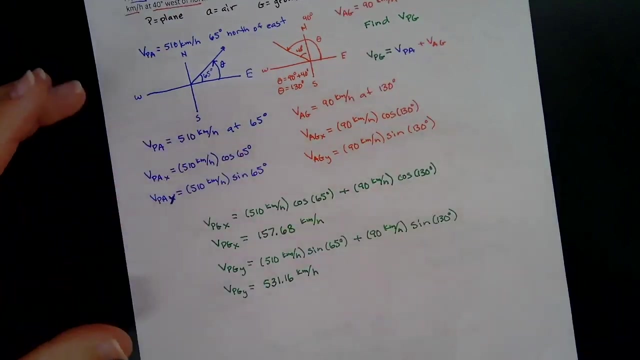 Okay, 510.. Sine of 65.. Plus 90 sine of 130.. And we get 531.. And we get 531.16.. And that would also be kilometers per hour. Okay, so we hit. now. we have this horizontal and this vertical component. They're both positive, right. 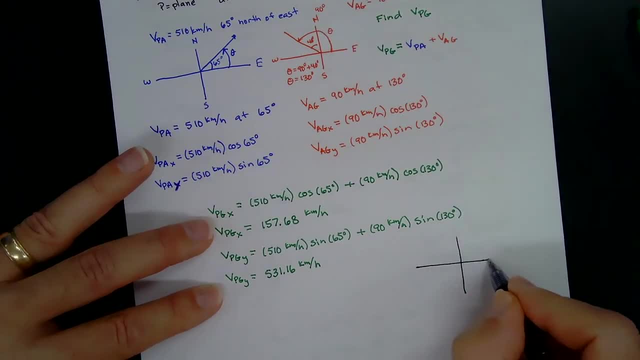 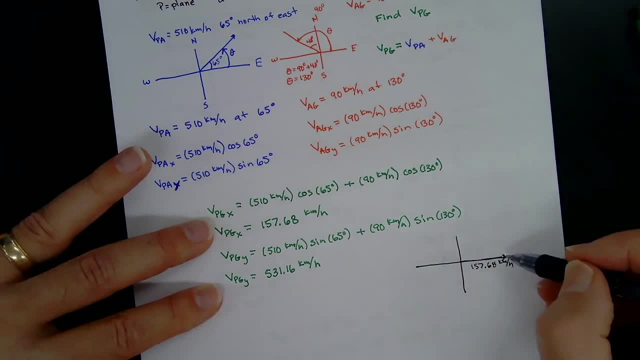 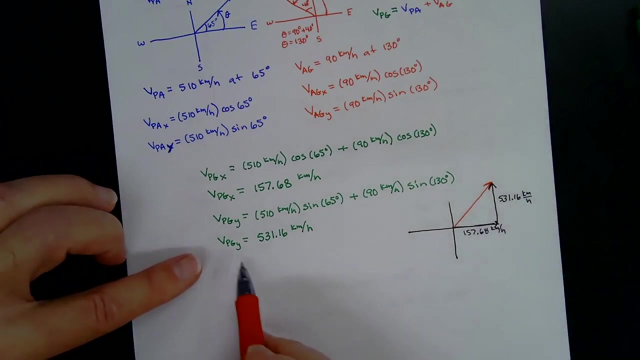 kilometers per hour, And I'm going to go up 531.. .16 kilometers per hour, And so my resultant vector is going to be in this direction. Okay, so now this would be my visa PG. it'd be this: this would be my V sub PG. it'd be this: this would be my V sub PG. 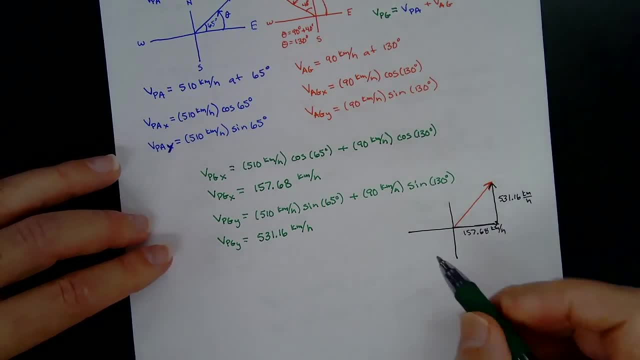 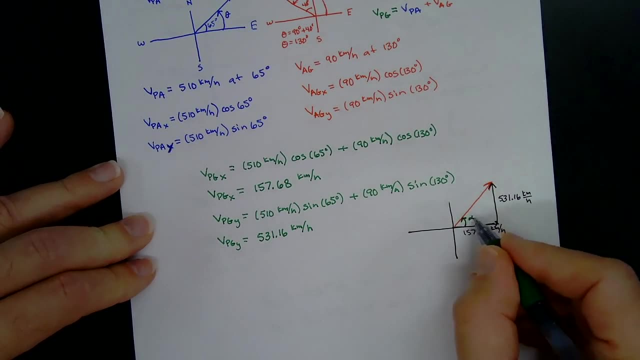 this would be the velocity of it. And then I got to also find the angle. Now, this is going to be nice, because my angle right here- okay, is my angle alpha is also going to be equal to my angle theta. So let's go ahead and let's do the. let's do the magnitude of it first, Okay, so v sub. 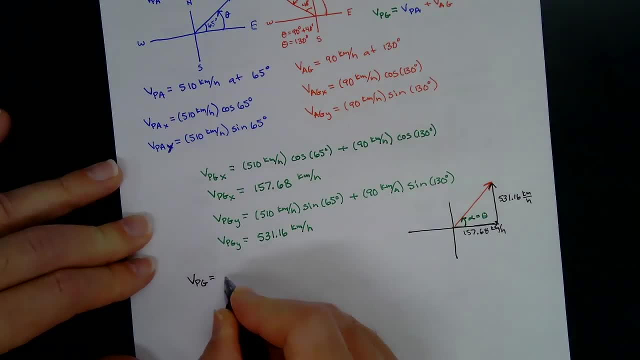 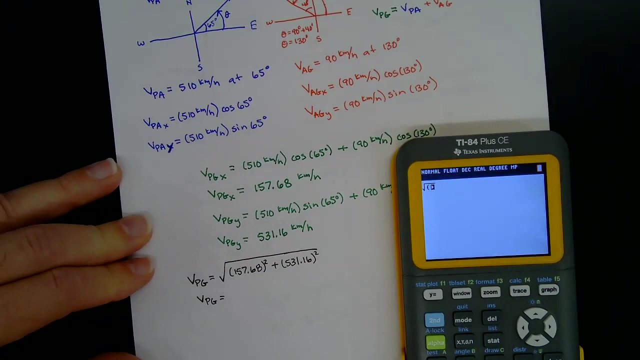 PG is equal to the square root. we're just using Pythagorean theorem here- and it'd be 157.68 squared plus 531.16 squared. So that makes the magnitude of this vector and square root and parenthesis- 157.68 squared plus 531.. You wouldn't actually need parenthesis for this one. 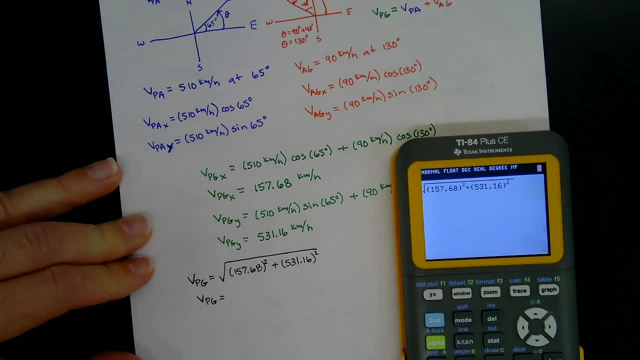 It's just I'm doing, out of habit, squared and we get 554 kilometers per hour. Okay, 554.1.. So this one, I'd like you to round the magnitudes, these horizontal and vertical, I want you to round to. 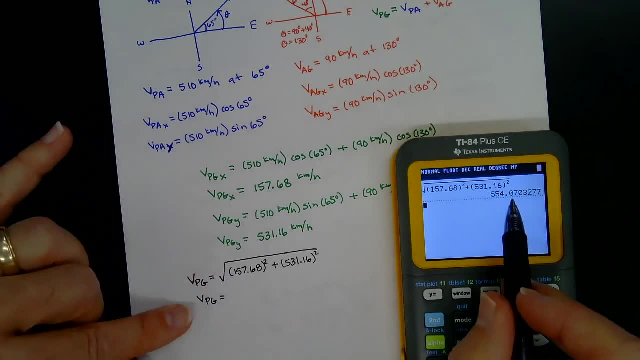 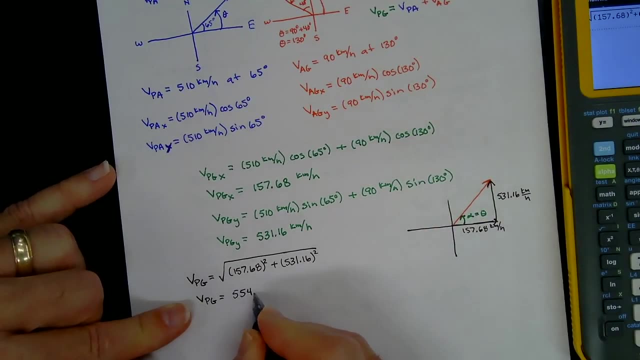 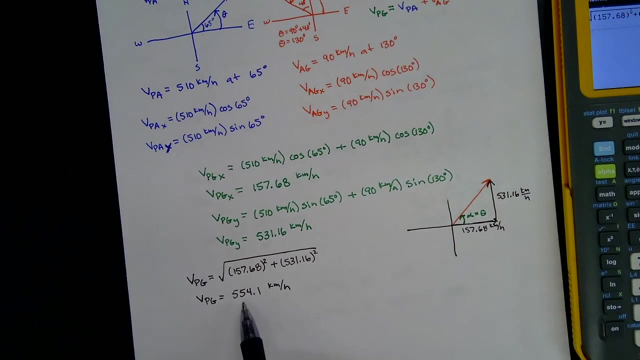 two decimal places And for the final magnitude, I want you to only round to one decimal place. Okay so, 554.1 kilometers per hour. So the plane was an airspeed was 510.. Right, So the air is actually causing it to go faster, Right, That's what this is telling me. it's going faster than 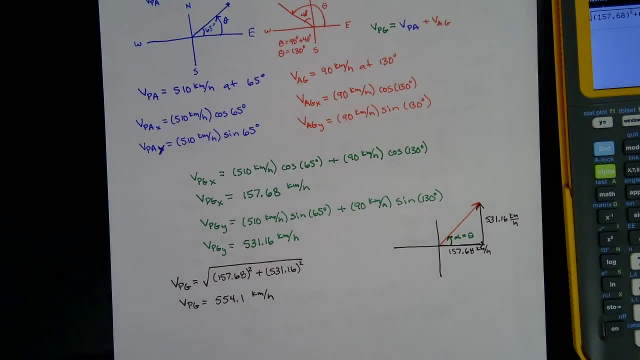 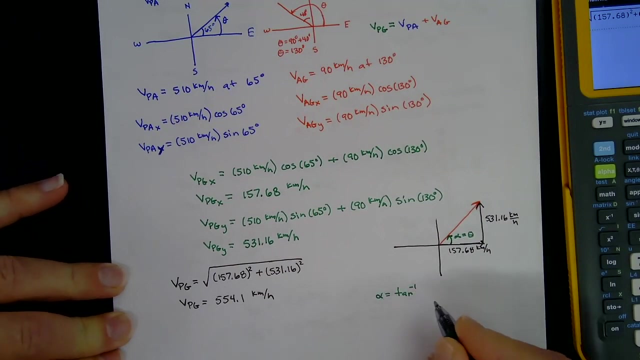 than just going without the wind. Okay, All right. Now, what direction is it going to go because of this wind? Right, Because it's not going to go the same direction it was going. Okay, so we got to get our alpha, and our alpha is tan inverse of, and it's gonna be the vertical piece. 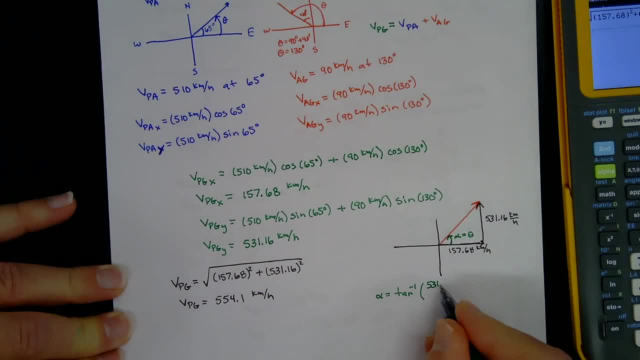 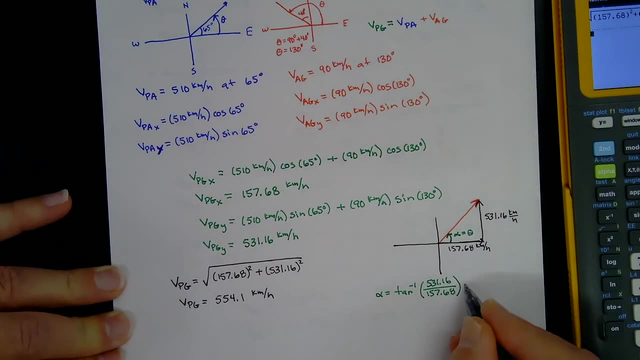 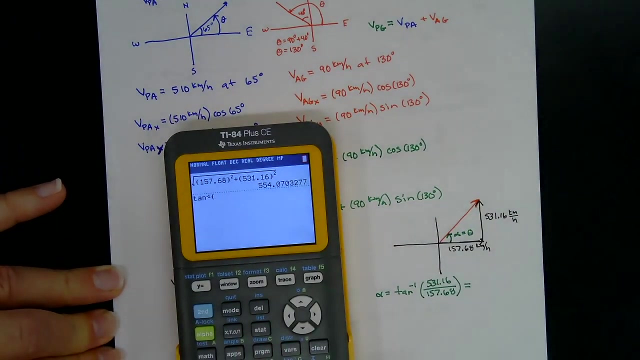 which is 531.16 divided by 157.68.. Okay, and this for angles. I want you to round to the nearest degree. So we're gonna press second tan And I'm gonna use a fraction bar here, So 531.16.. 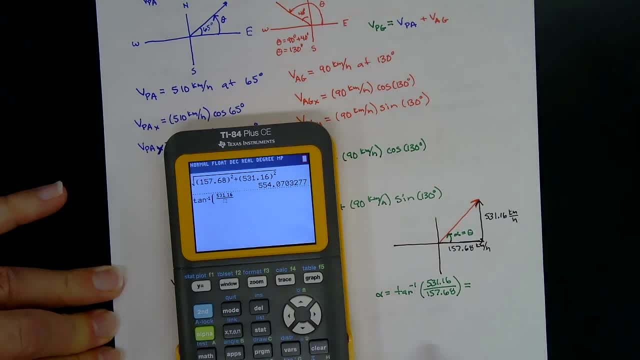 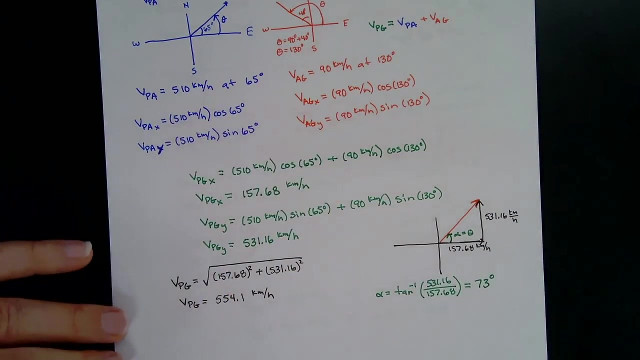 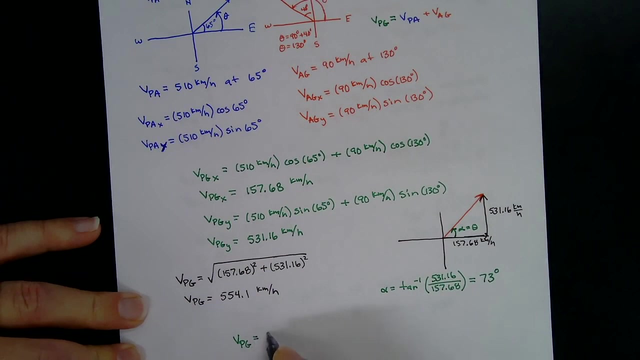 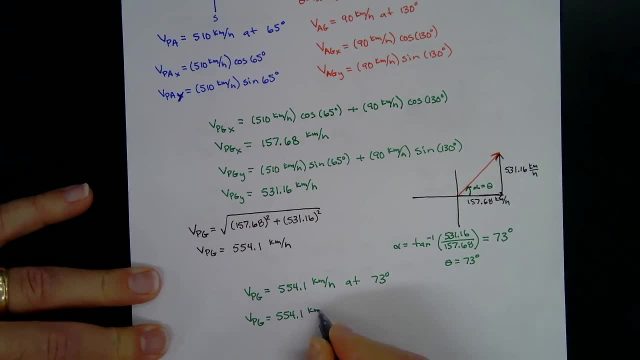 Okay, so we know V sub PG is equal to 554.1 kilometers per hour. Okay, so we know V sub PG is equal to 554.1 kilometers per hour. one kilometers per hour and it's going to be 73 degrees. we're gonna have to rotate 73 degrees. 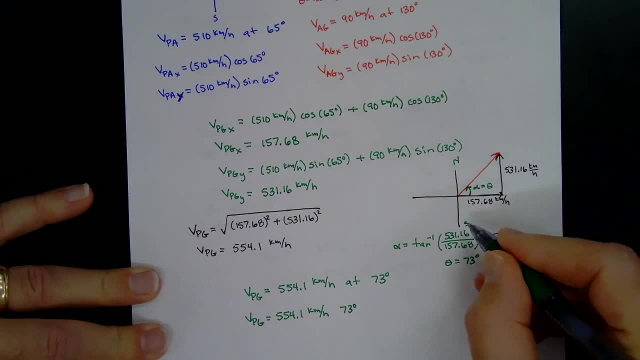 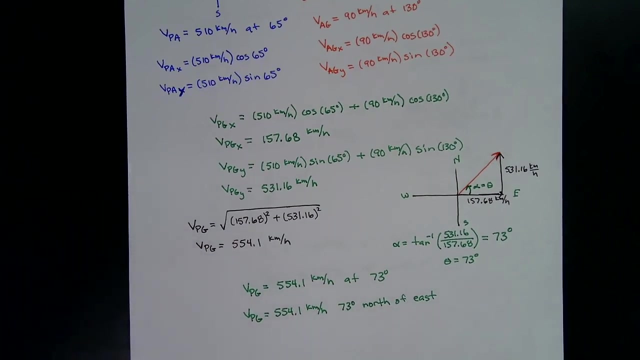 and this is north and this is south and this is west and this is east. so we're gonna have to, from the east we're gonna have to rotate towards the north, so that'd be 73 degrees north of east. okay, so i know that it's like man, that's a lot of calculations. i, i get, i get it, but really 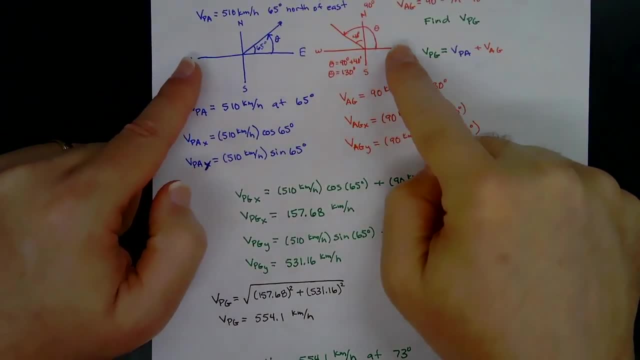 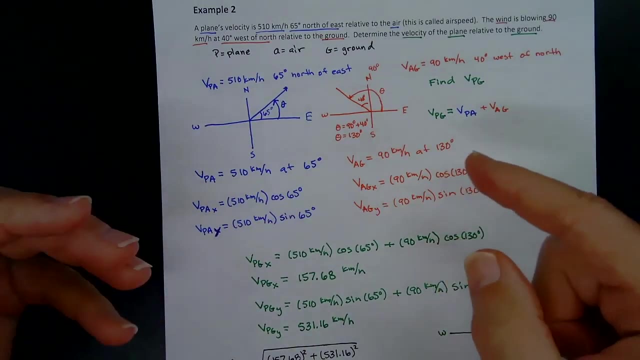 the. the idea is, you got your two vectors right. you got to get the horizontal and vertical. well, you got it, if they're written in the description form. you got to get the angles right. so you got to get the angles and then, from there, get the horizontal and vertical components of each. 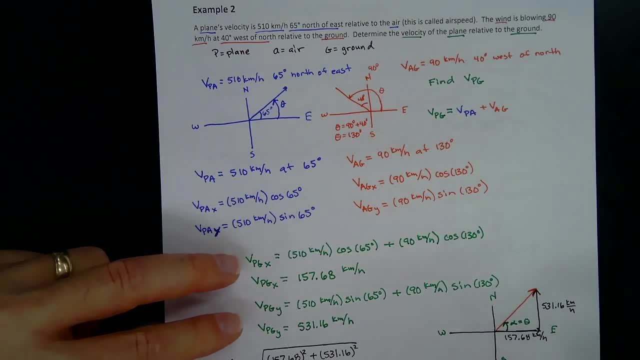 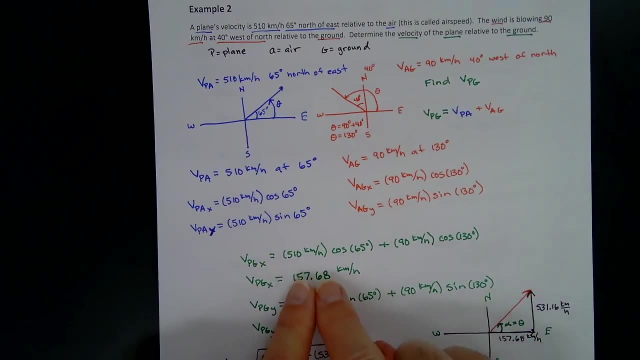 and then you got to get the angles right. so you got to get the angles and then from there, for our resultant vector- okay- which in this case is v sub pg- we need to add these two horizontal components and that's going to be our new horizontal component. we're going to take our 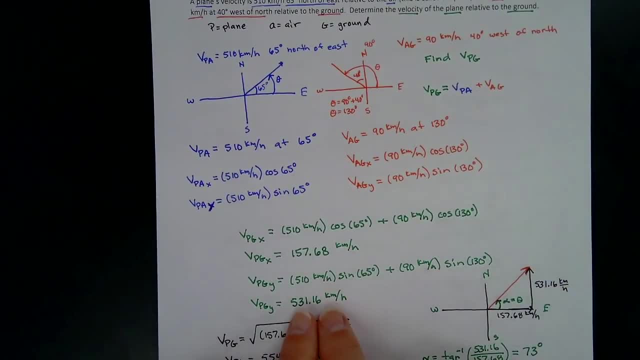 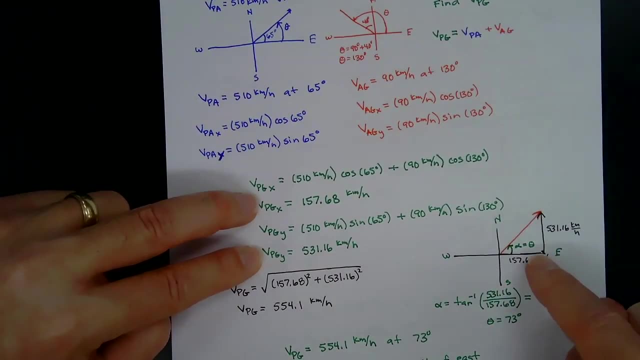 two vertical components and we're going to add them and that gives us our new vertical component. and now, because we have these horizontal and vertical components, i can draw a diagram with those and know the direction i'm going to go right. and then i can find the magnitude by just 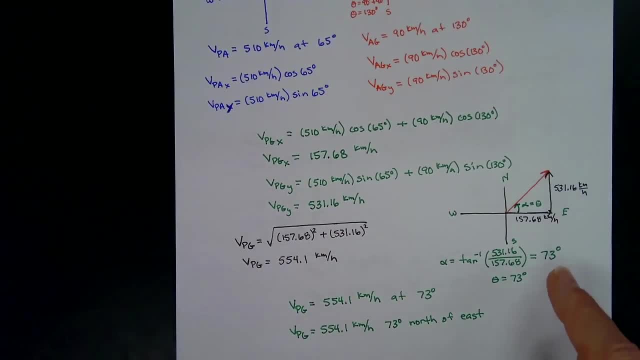 pythagorean theorem: okay, and then i can get the, the reference angle or the angle of the triangle, by taking tan inverse of this over this and then, depending on where, this is, okay, if it was in this quadrant or this quadrant, or this quadrant, right, you're going to have four different directions. it could go. 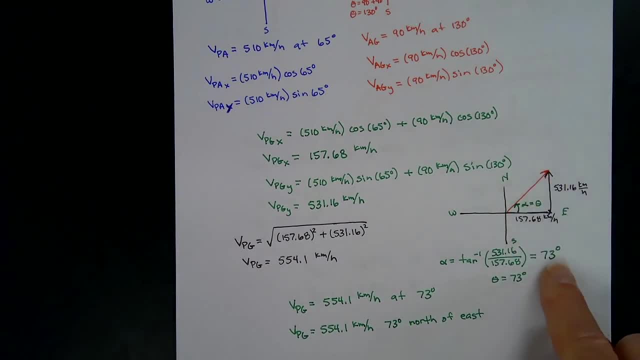 okay, but because it's going, this one, the, actually the, the direction angle and the angle, the triangle turn out to be, in this case, the same angle: 73 degrees. okay, all right, you guys, that's it. 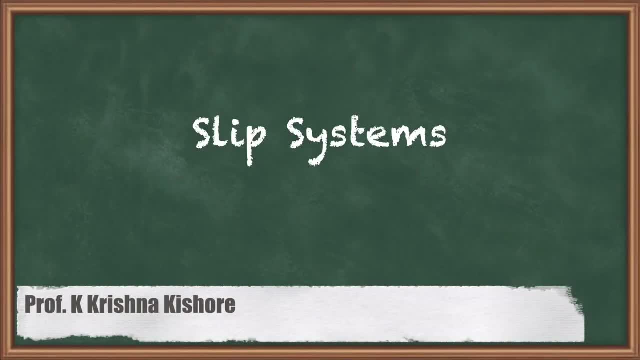 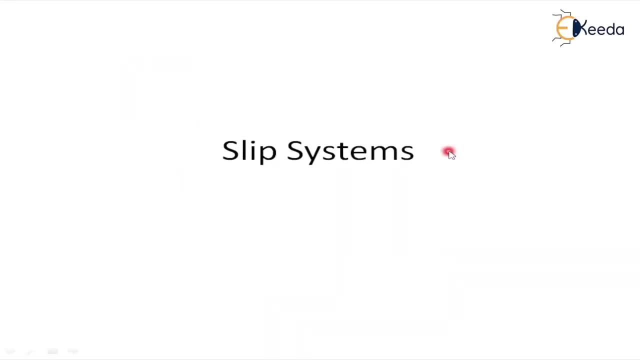 Hi, I am Kakarla Krishnageshwar, Mechanical Engineer. Today we are going to discuss slip systems in material technology. Now, in this session, we are going to discuss what is slip system and the various types of slip systems in material technology. 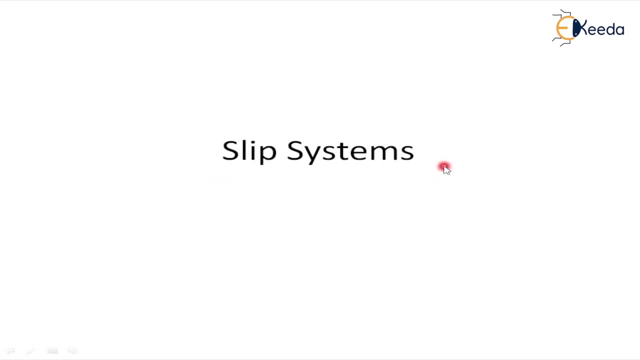 The slip systems plays a vital role in deformation and in understanding material properties. If the slip systems are able to understand in a proper manner, we can assess how much deformation may be existed in materials. Let us discuss the various slip system and the salient features in slip system. 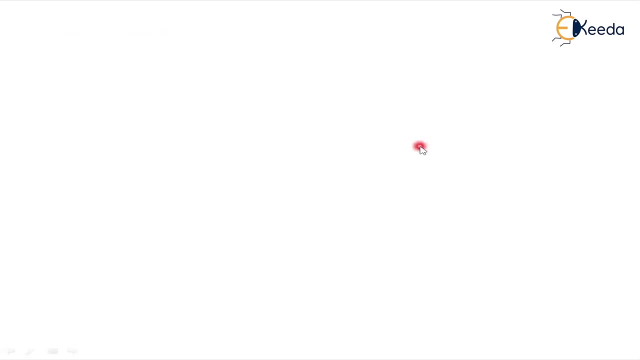 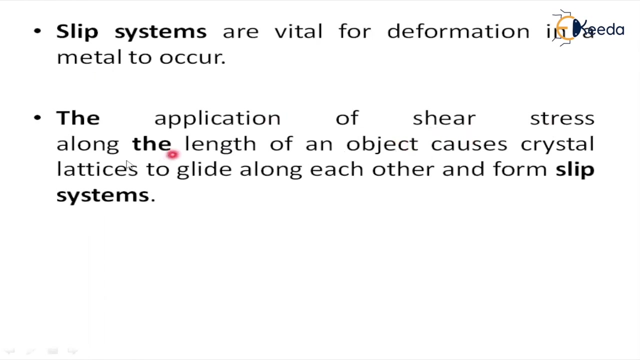 Let me discuss like this Now. the first one is: the slip systems are vital deformation in a metal to occur. This is the first. The second is the application of shear stress along the length of an object causes crystal lattices to glide along each other and form slip systems. 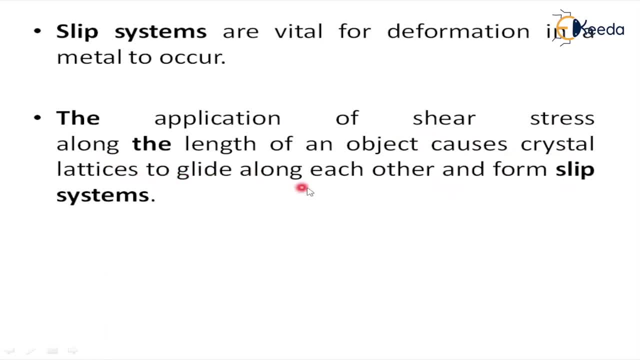